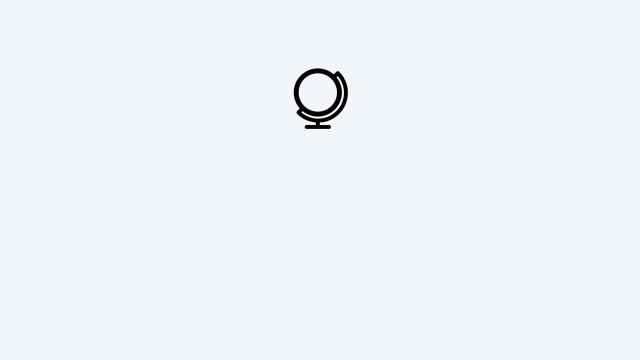 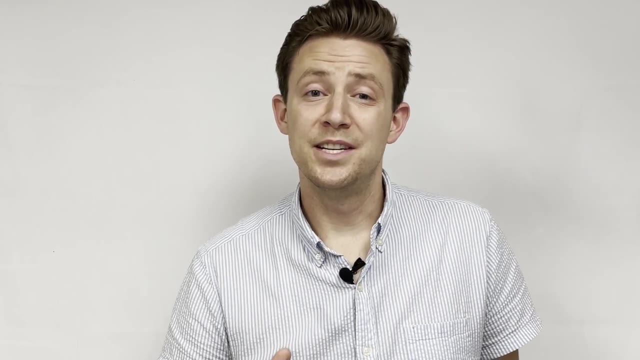 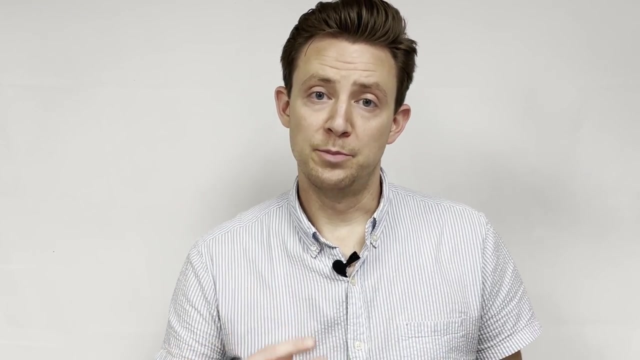 So with that, let's jump right in. Hi everyone, my name is Matt Forrest and today we're going to learn the most important tools that I think you need to get started with modern GIS in 2022.. This is not a comprehensive list, but I think these are the things that, if you start with, you can start to build a really good foundation and grow your skill set in multiple different areas, depending on where you want to start. 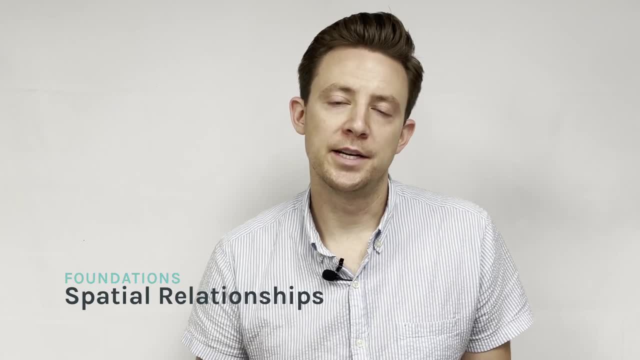 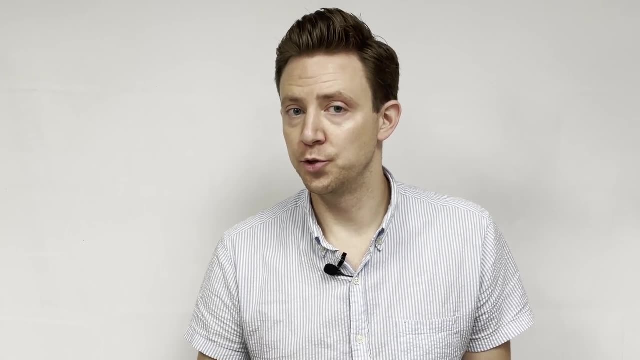 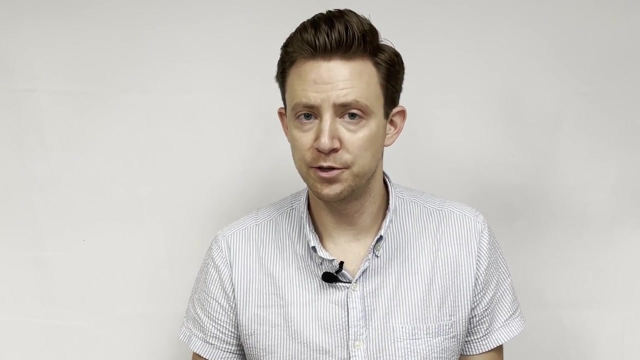 So the first area to focus on is some fundamental GIS concepts. Now, if you've gone through a GIS or geospatial education, you've probably studied these things before. Things such as spatial joins, how spatial features touch each other and interact, measuring distances, nearest neighbors, so on and so forth. 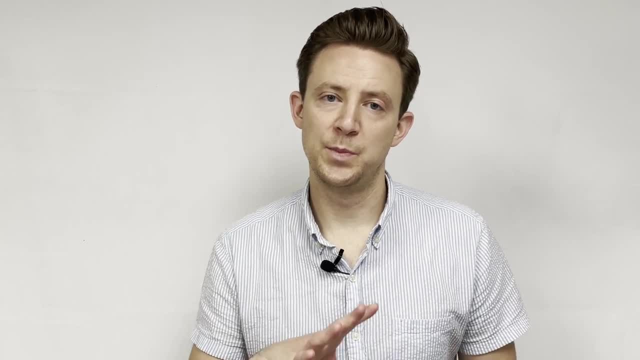 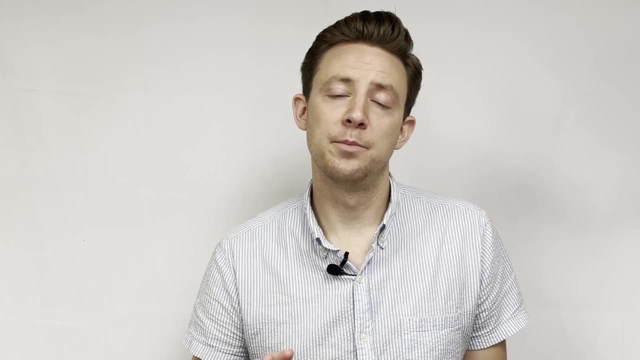 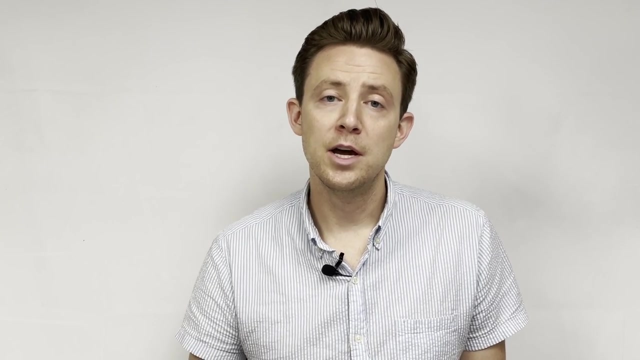 This happens to be one of the things I do. most of my job is using spatial data, combining it using spatial interactions and spatial relationships. So this is probably the number one topic I'd focus on and I'd pull away from a traditional GIS. Now, how you do this with different technologies, we'll talk a little bit more about later in the video, but that's one place to start. 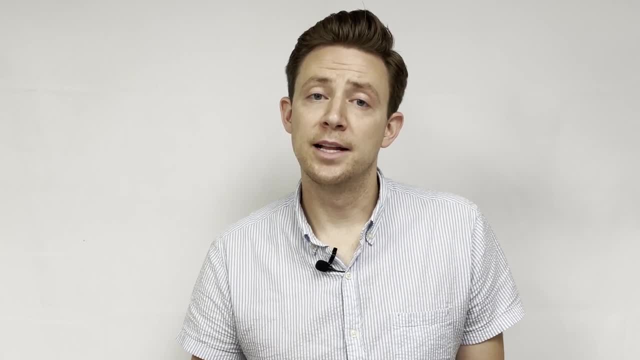 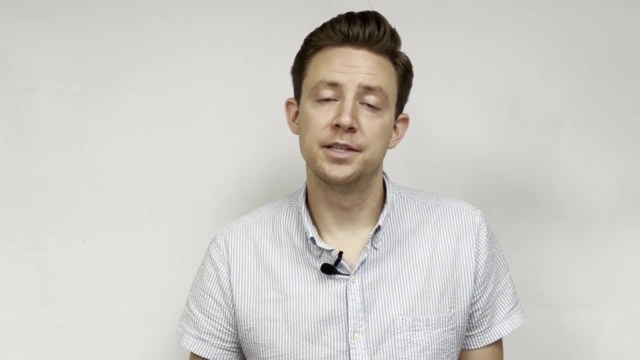 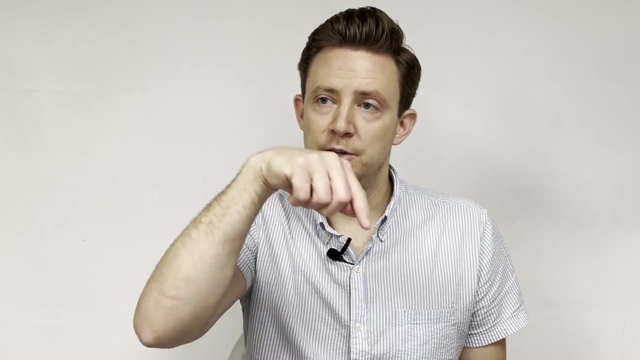 A really important example of this is exploratory spatial data analysis, or ESDA. There's a Python package from PyCell where you can actually use and implement that Effectively. what this does is perform an analysis called spatial autocorrelation or Morin's eye, and it looks at a specific feature and the features surrounding it, the ones that touch or have different spatial relationships. 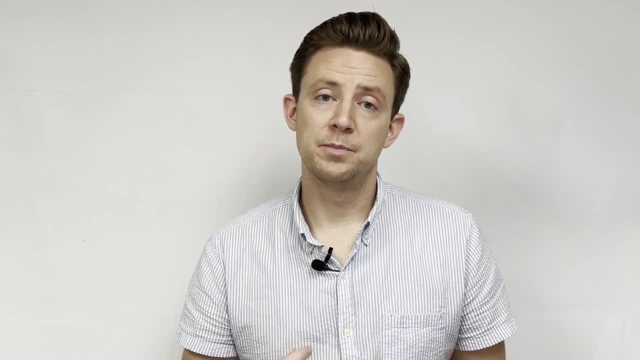 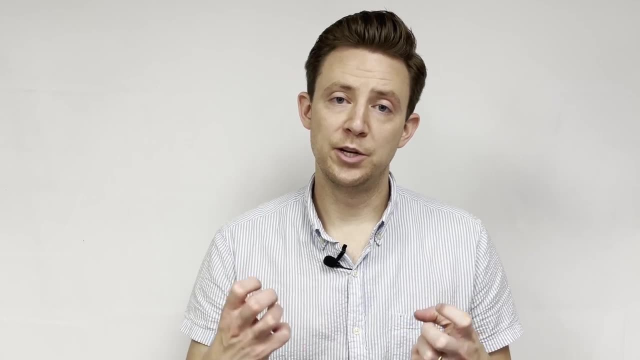 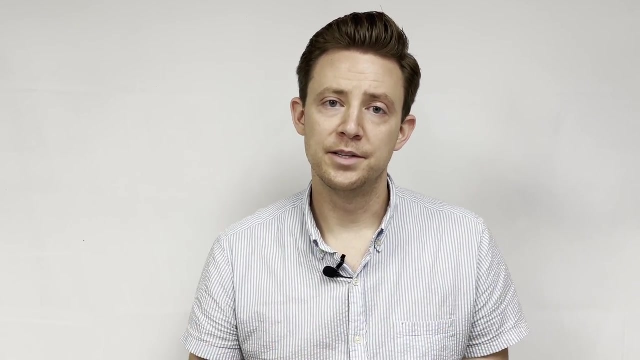 There's lots of different ways You can actually do this. in the package They call this spatial weights and you can take a look at that in this link over here Now. using this, you can actually evaluate the spatial clusters or spatial relationships using some statistical methods, and that same analysis can apply to lots of different areas. 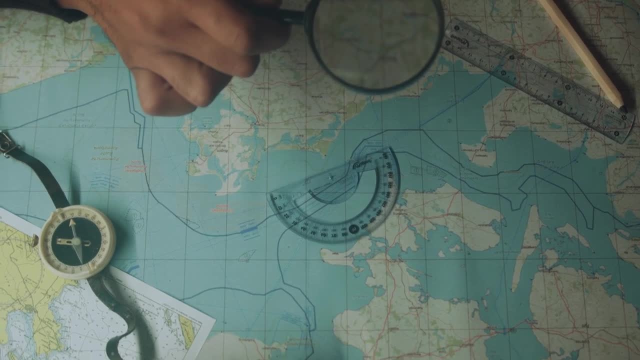 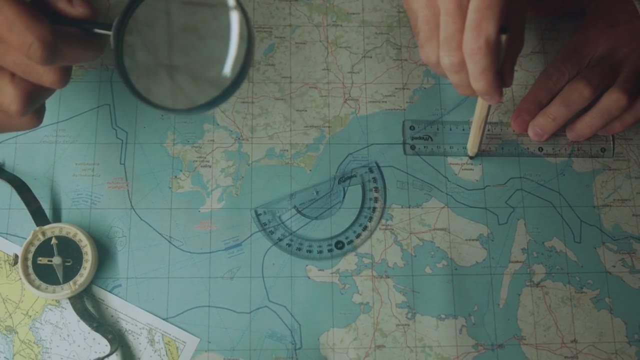 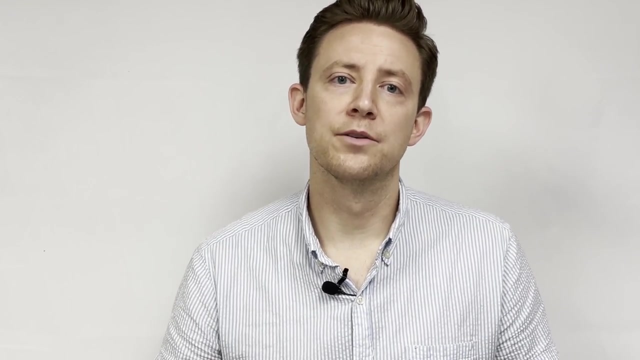 So really understanding how to use spatial relationships is a very important concept in modern GIS. Other concepts I would definitely take a look at are using other data to create geospatial features. Things like geocoding addresses is really important. It can get really complex if the address data is not clean, clear or consistent. 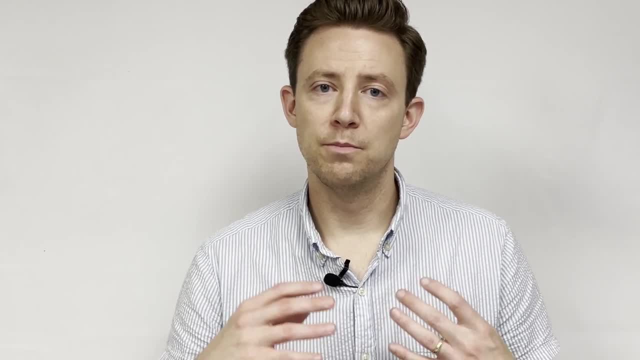 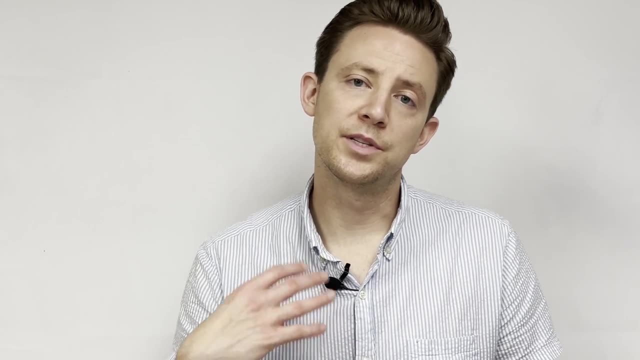 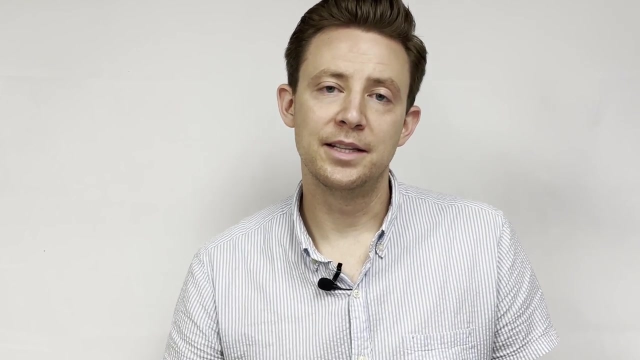 Also understanding the concept of trade areas, where people might go to certain places or interact with certain things. Now, you can do this multiple different ways. You can use a simple radius, You can use a concept of an isochrone or a drive time, or you can use human mobility data to calculate these. 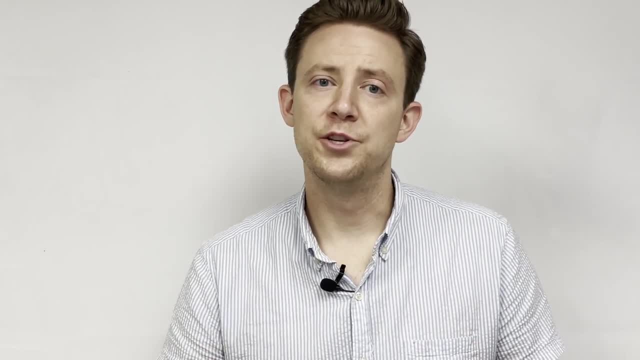 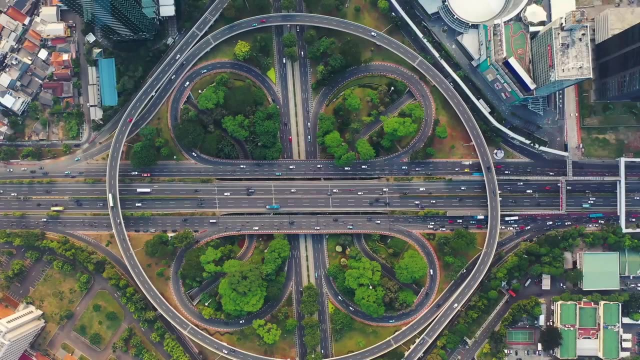 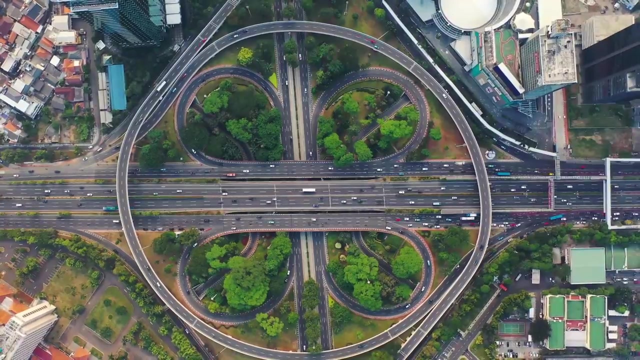 But having an understanding of how you define a trade area and how the features interact with that data is very important as well. The last piece I would also Work on understanding is network analysis. So understanding maybe it's a road network, maybe it's things like rivers, other features like utility lines, all encompass network analytics. 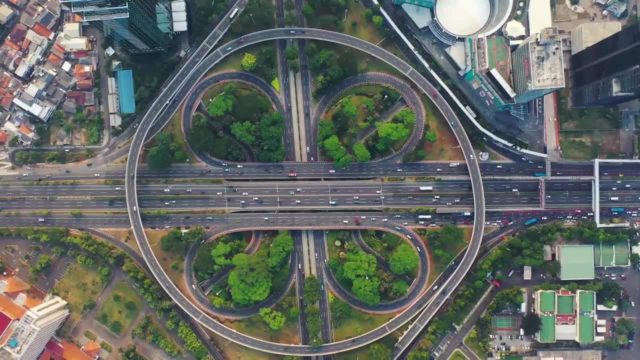 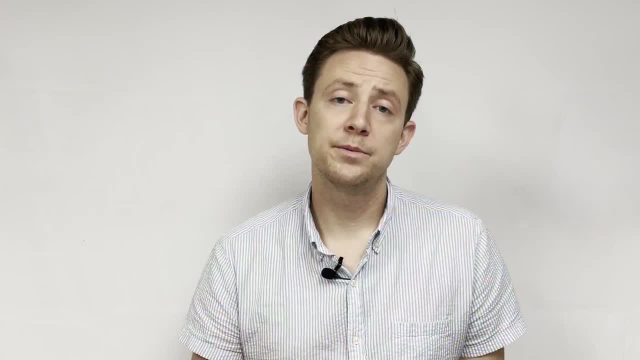 There's great tools for this as well. We'll talk about that a little bit more later, But understanding the basic concepts of network analytics is also really important. Now you'll notice that I didn't cover some concepts from a traditional geography education. 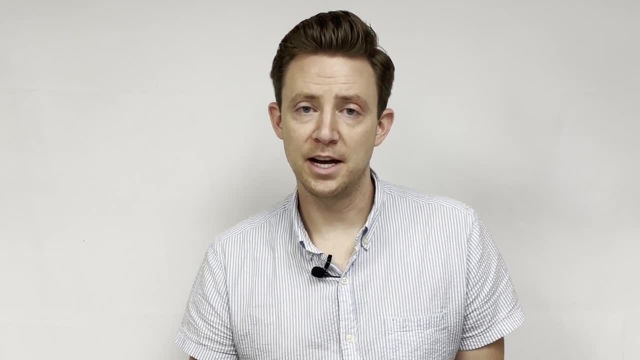 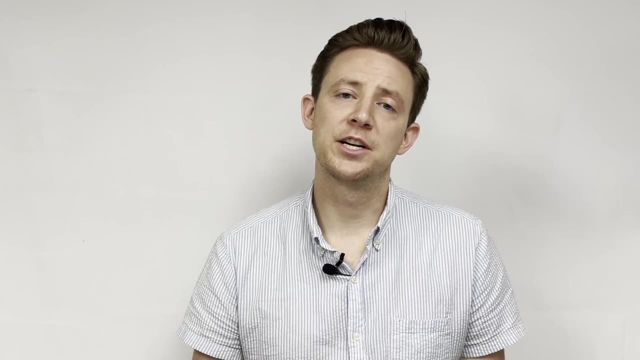 Things like map projections, some basic cartographic concepts and all these different pieces. As it relates to map projections, I would say the majority of analysis really happens in a handful of projections, So having some basic engineering to get into those projections is going to be important. 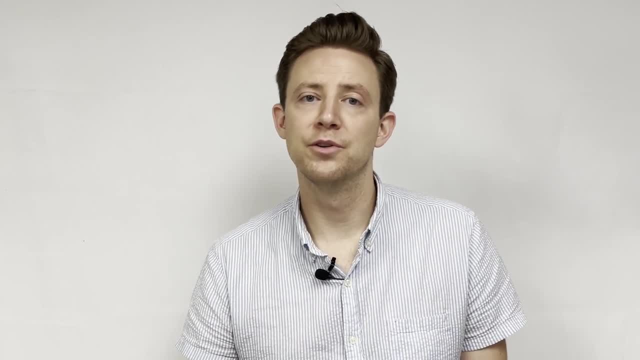 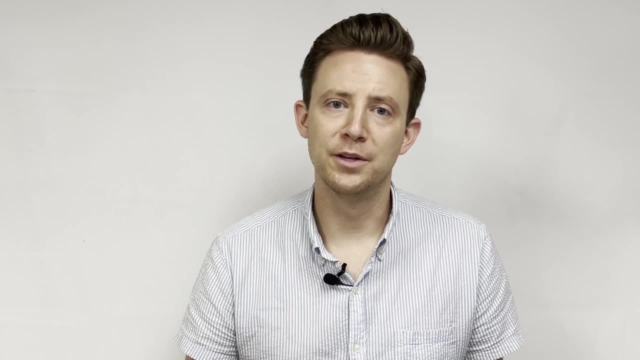 But understanding all the dynamics of projections is not as critical in modern GIS as it relates to cartographic design. You might want to know how to use a Jenks break or equal intervals or some other geographic cartographic design concepts, But it's not as important in modern GIS. 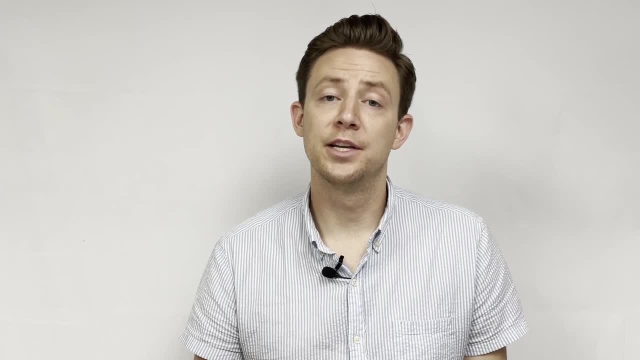 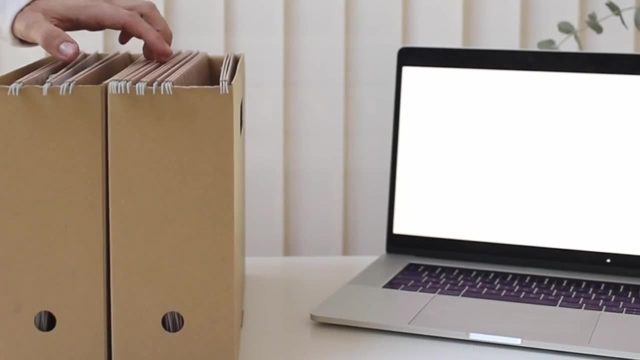 There's great tools to do this And we'll talk about that In the visualization section later in this video. Now, if you work with geospatial data, before you know it comes in lots of different shapes, sizes and, most importantly, formats. 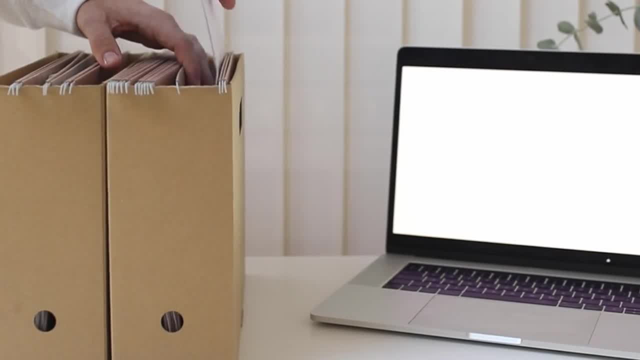 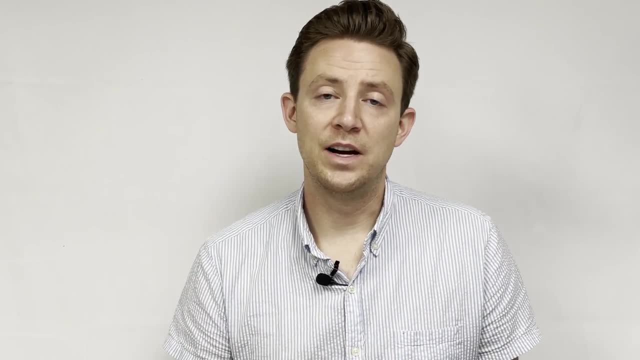 And I'm not just talking about the difference between raster or vector data. I'm really talking about all the different file formats that you can use in those two data types. We all know the common ones, like shapefiles, GeoJSON, CSVs, even into KMLs or other file types. 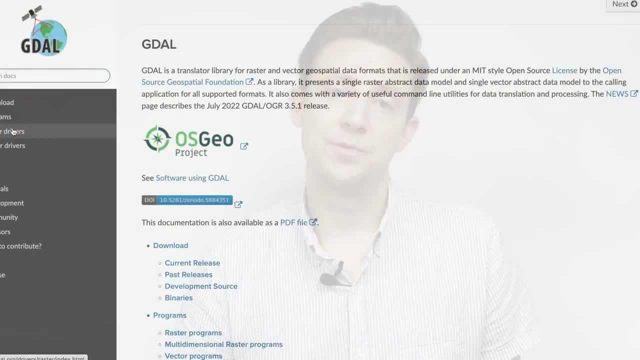 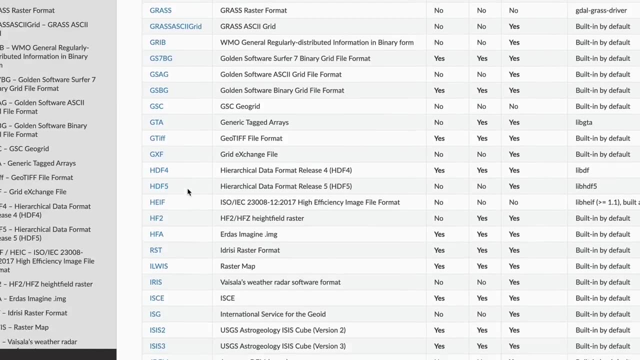 But there's a whole list- almost 200 different file types across raster and vector data sets That you can actually store geospatial data in. There's a number of reasons for this, And we can maybe talk about that at a different time. 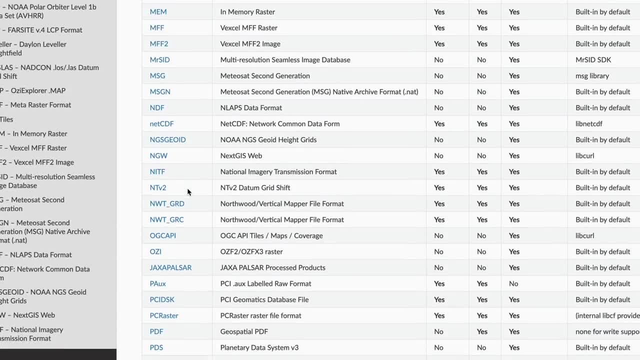 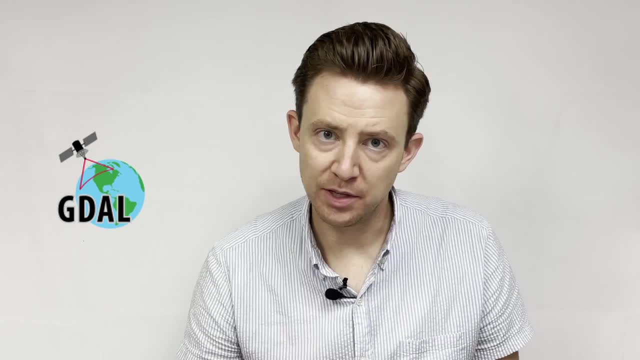 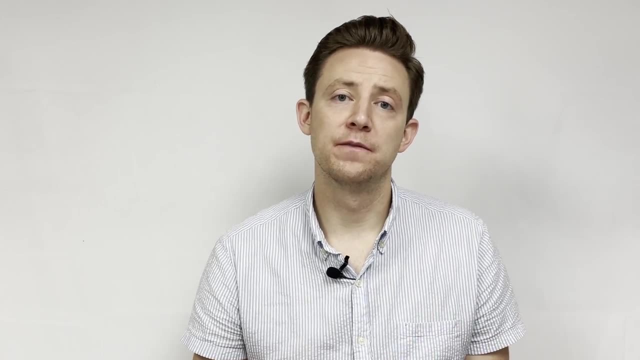 But you need to be able to move that into the file type that works best for you. What's the best tool to do that? GDAL. GDAL is a base library that's mostly written in C++. That's incredibly fast and has multiple drivers to different libraries like Python or others to actually use in different settings. 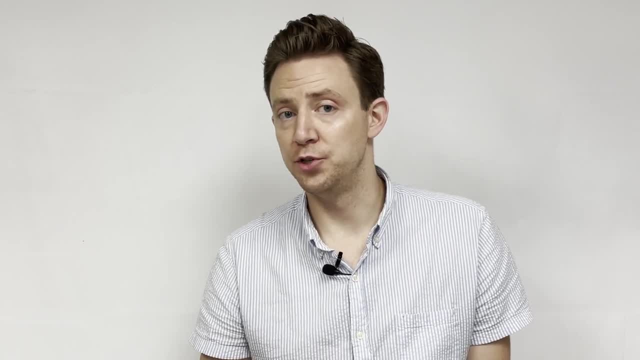 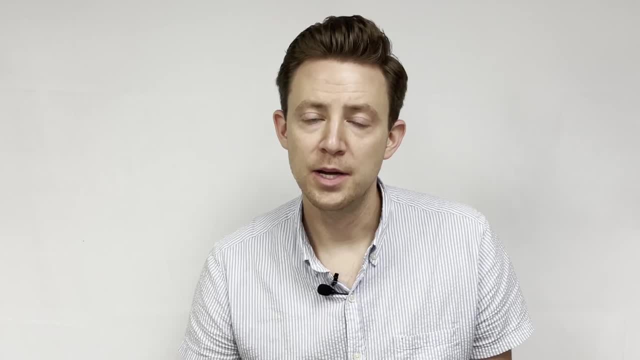 It's embedded in many of the tools you use, such as QGIS, GeoPandas, etc. It's embedded in many of the tools you use, such as QGIS, GeoPandas, etc. It is one of the most critical pieces of geospatial infrastructure that exist today. 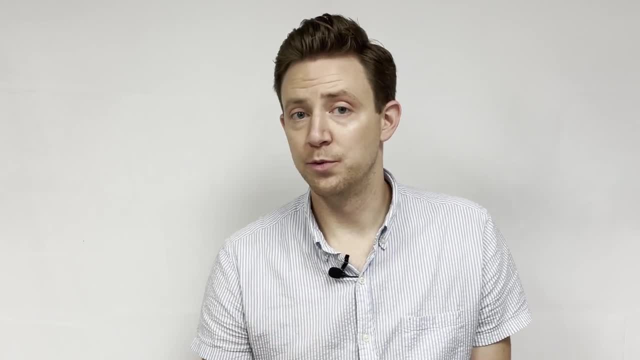 It is one of the most critical pieces of geospatial infrastructure that exist today. How do you make use of this? There's multiple ways. You can use it in a Python library. you can use it in one of those other tools that I mentioned. 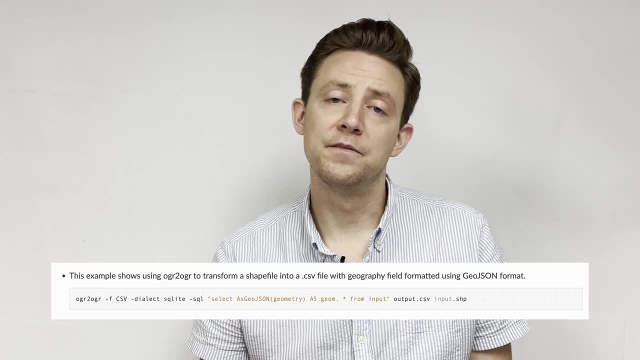 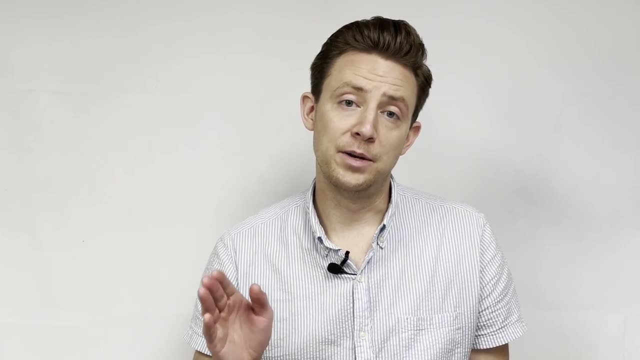 Or, as I use it quite often, you can use it directly on the command line of your computer. There are some installation instructions, depending on your operating system, which you can check out, But I highly recommend putting some work into this. Why. 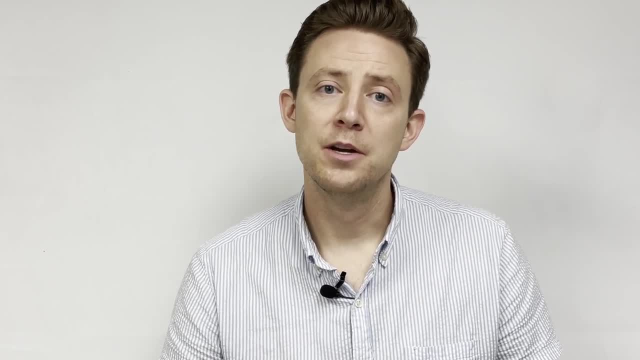 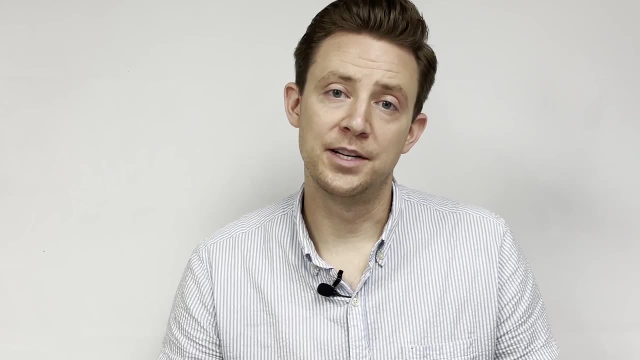 It can solve a lot of problems. There is a wide array of data engineering problems for geospatial data. Let's say you need to change a projection- Use GDAL. Do you need to rasterize or vectorize some data? Use GDAL. 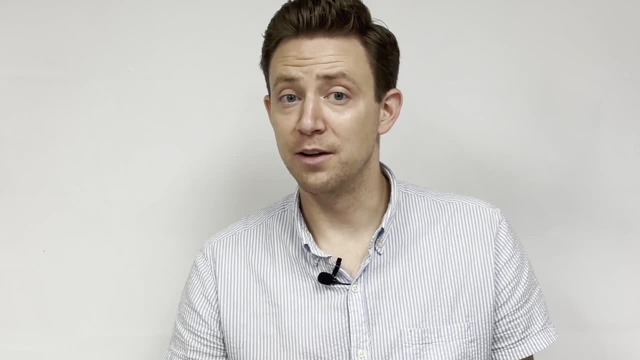 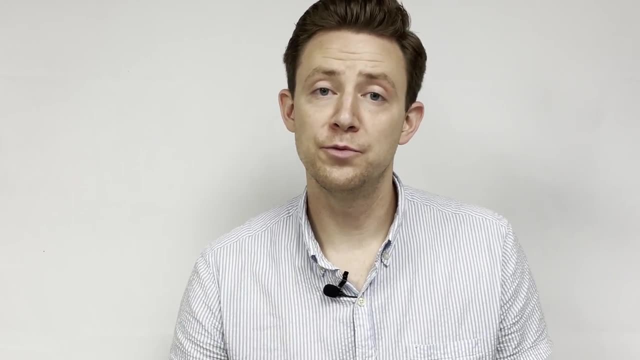 Do you need to manipulate geometries? at a very base level, You can use GDAL. Do you need to abstract some data, to add a different geometry type column, maybe in GeoJSON, to import into a different tool? Guess what? You can use GDAL. 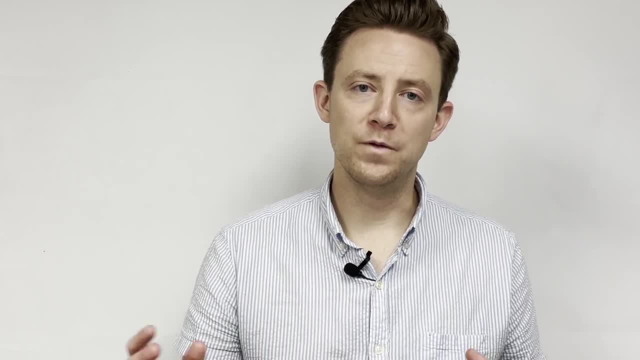 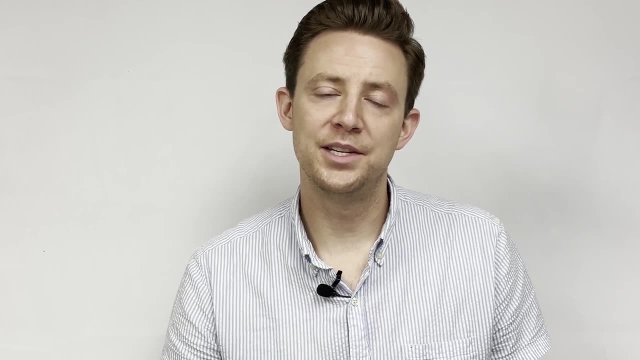 GDAL covers so many wide ranges of use cases for moving and manipulating geospatial data- manipulating geospatial data- that is just worth investing some good time into practicing with that library and using it for these base geospatial data engineering problems. Now there are some. 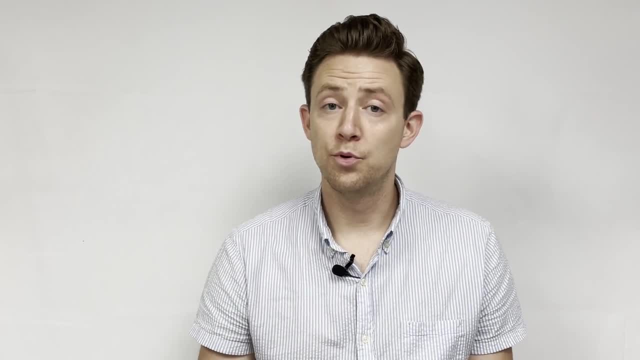 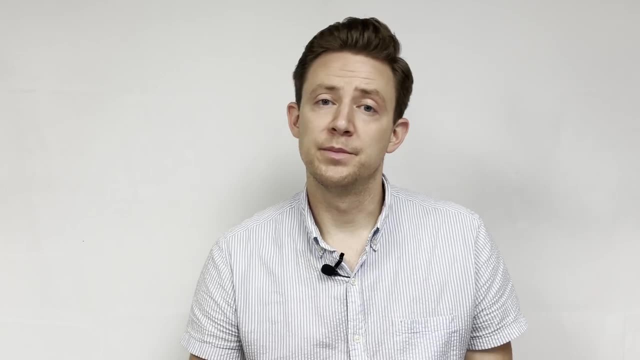 other basic geospatial data engineering concepts that I think are important, Things like using unions and aggregating data. also using and manipulating data to move into different systems like a database or data warehouse. GDAL can help with a lot of this, So keep that in mind as you're. 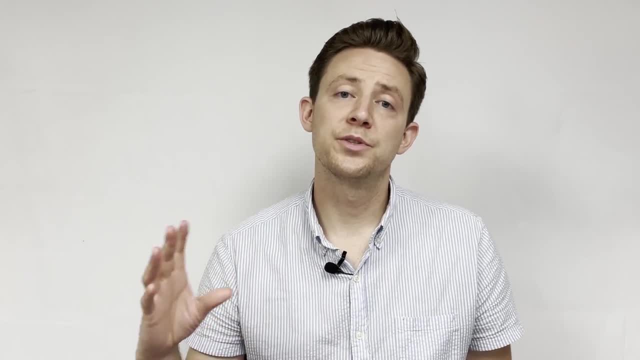 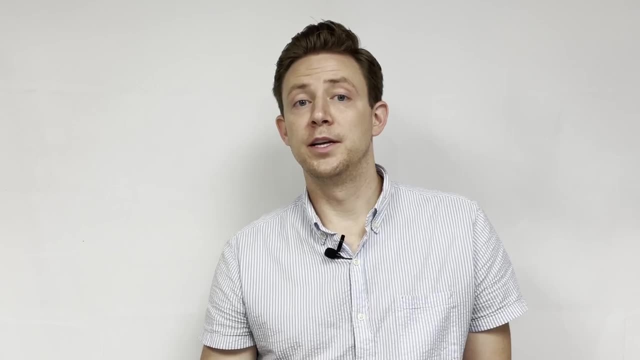 going along, And we'll also talk about the importance of spatial SQL in geospatial data engineering in a later section, But for the most part, GDAL is going to be your core toolkit for doing and solving a lot of these problems. The last piece I want to touch on was spatial indices. 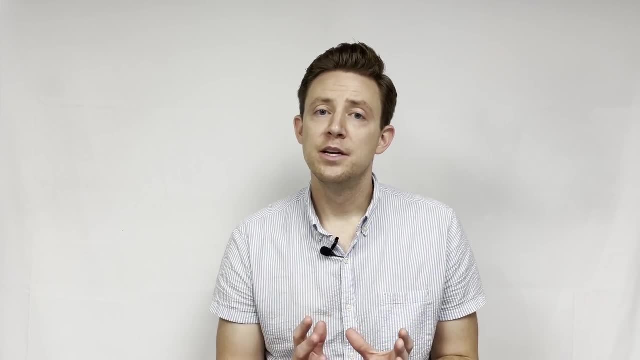 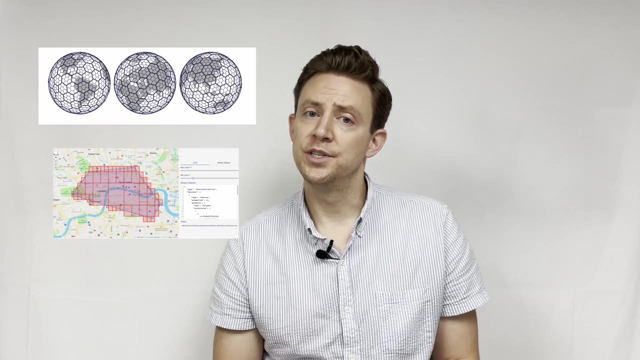 Now, a spatial index is effectively a geometry, but that is stored in a string or a numeric format. Now, some examples of this are H3 cells, S2 cells and quad bins or quad integers. These are really important for storing data. So if you're doing a lot of work, you're going to want to have a 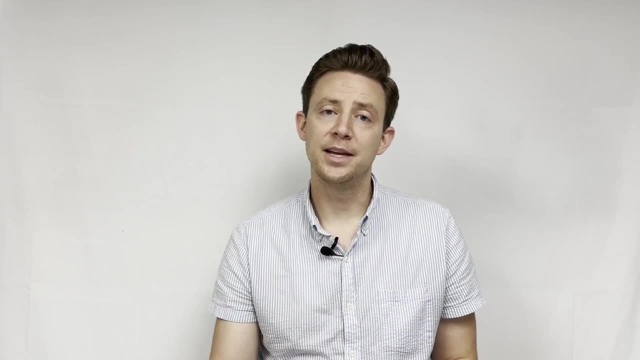 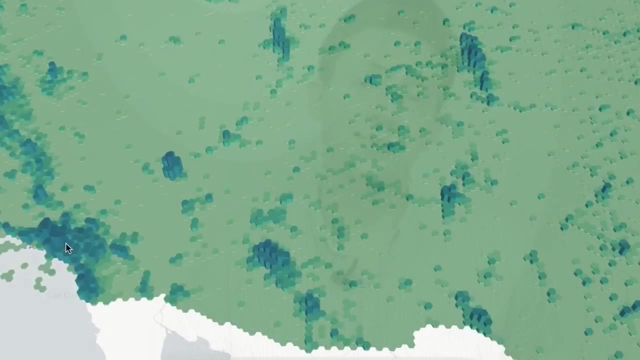 large data- set in point data- and making it very easy to quickly aggregate and then visualize that data in other different tools. Now, as you see in this map, as I zoom in and out, you can see the cells and the aggregations are changing. The data that's underlying this map is actually point data. 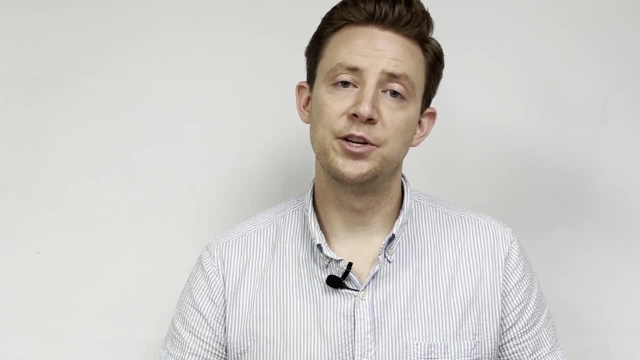 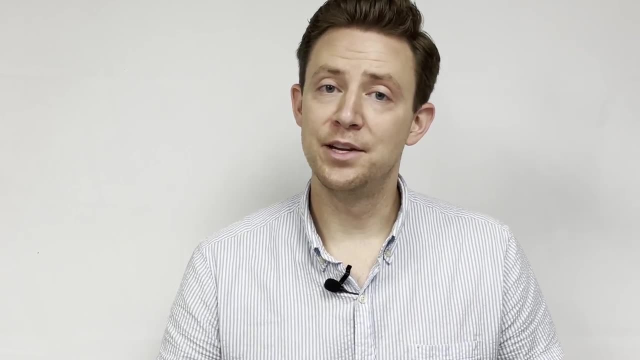 So what I'm doing is effectively joining that and using these spatial indexing systems- in this case H3, to actually aggregate this data. But when I'm visualizing the map, I actually am not using a geometry, I'm just using that H3 data. So what I'm doing is I'm actually using that H3 data And 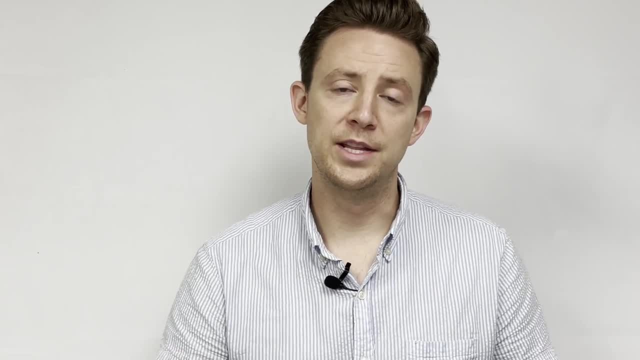 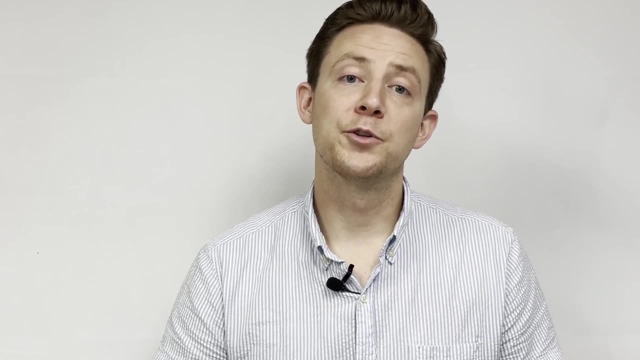 I'm actually using that H3 string index to join that data to the front end and visualize it. that way, It's incredibly efficient for storing and querying data, And we'll talk more about that in a future video, But this is one concept I want to make sure you know about. Now you can use spatial. 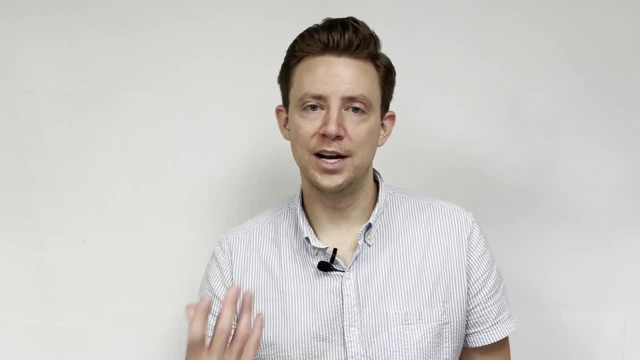 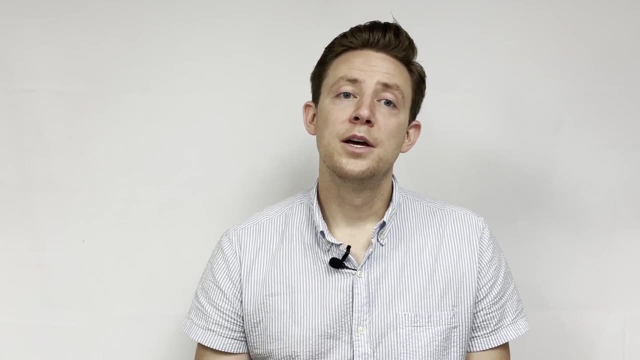 indices lots of different ways. There's libraries written in Python and JavaScript and others that you can actually use and leverage to create spatial indices. You can also use this through spatial SQL and can do that directly on a database or a data way. So if you're doing a lot of work, 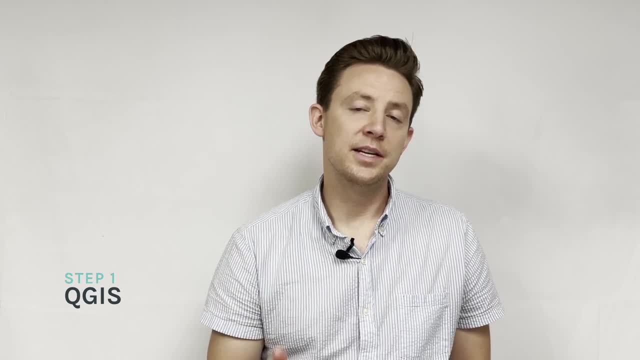 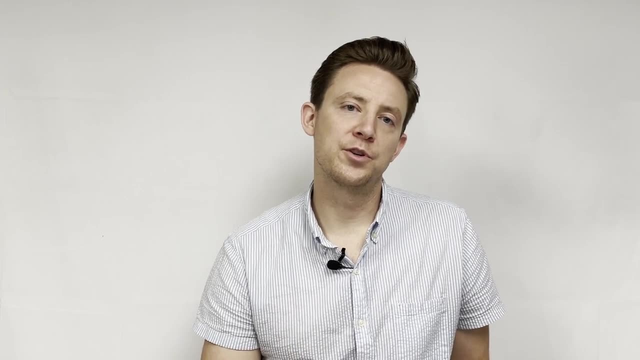 you can use this. You can use this to create a data warehouse. My next tool kit that I highly recommend using is QGIS. QGIS is one of the most indispensable and most important pieces of geospatial infrastructure for modern GIS. Now, yes, it is a desktop tool and you might be expecting 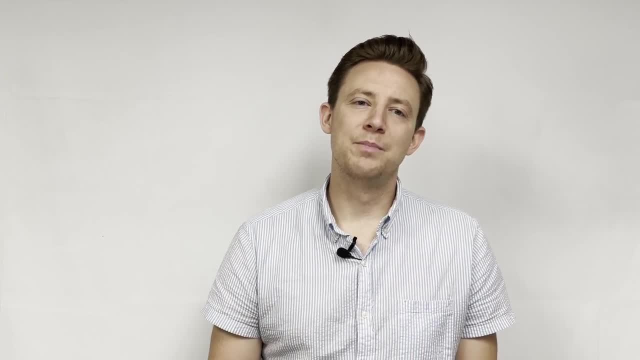 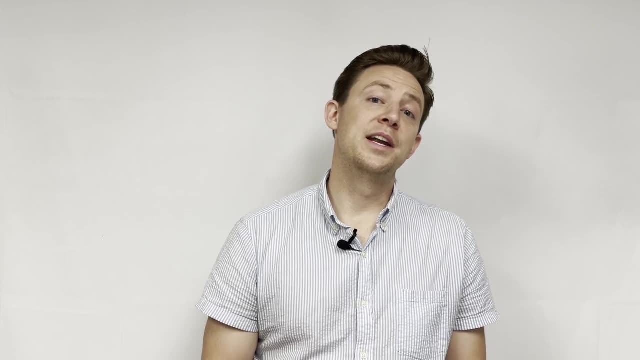 to me to talk about programming and computer languages and all these different things. But QGIS embeds and has so much of that and is very easy to start using and introducing yourself to the different components. On top of that, it has a rich ecosystem of plugins and other toolkits that you can use to create your own. 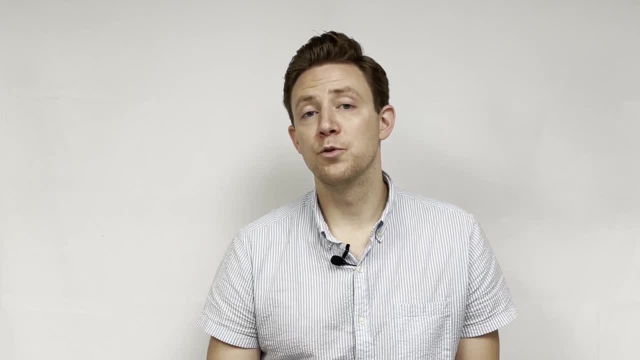 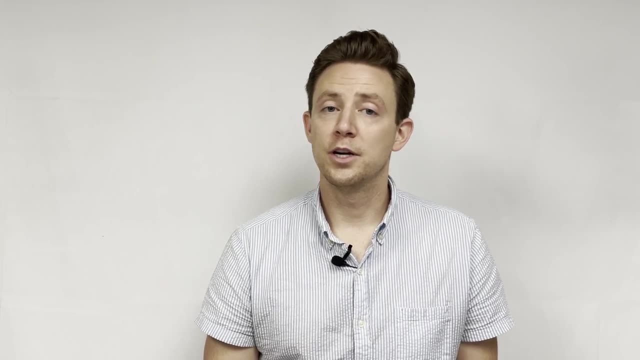 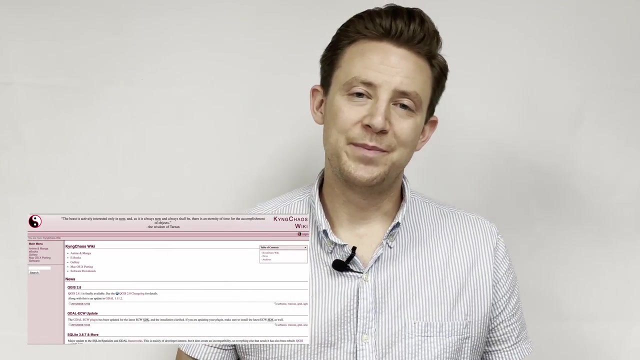 data. If you come from more of a traditional GIS background, this is a very easy introduction into using modern GIS tools and concepts, And we'll talk a little bit more about why that is in a minute. I've been using QGIS since around 2010, and it was a much different experience back. 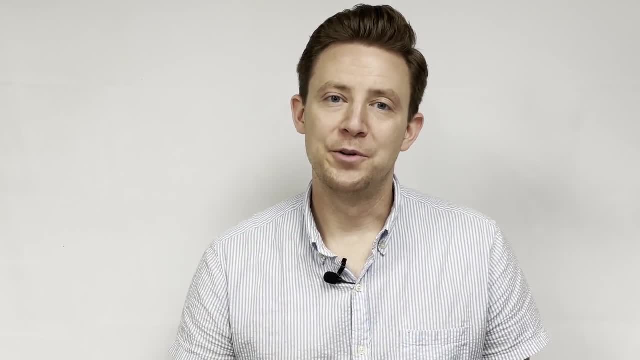 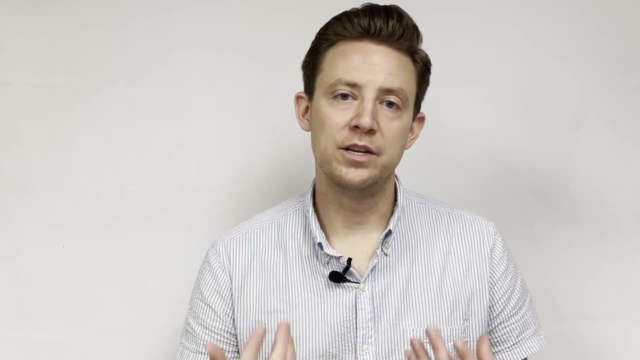 then in terms of downloading the software and using it. Fortunately, now in 2022, it's very easy to use it. get started. There's releases and communities and support infrastructure for actually using and learning this tool. One way I've talked a lot about QGIS is that it's very 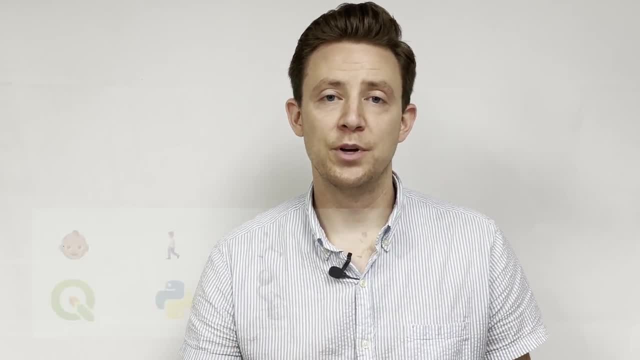 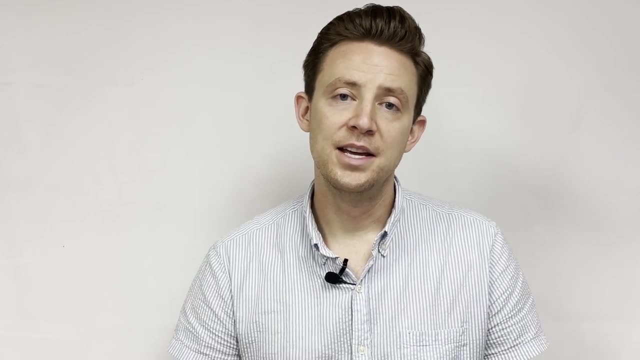 easy to use. You can download it and install it on your computer. You can do a lot of things. One way I've talked about learning modern GIS in the past is through a crawl, walk, run and then sprint process. QGIS is the first step of that process that introduces you to a lot of these different 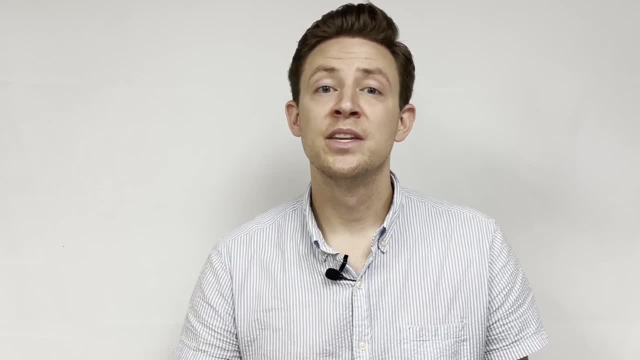 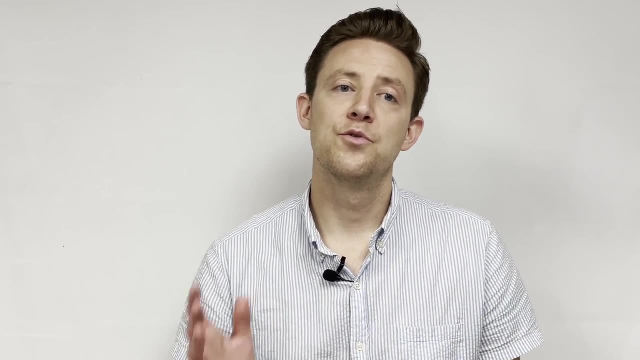 concepts. Now, one thing I love about QGIS is when you download it it installs GDAL for you to use and embeds GDAL and a lot of the data abstraction processes and data engineering tools within the platform itself. There's so much you can do with QGIS that's hard to mention here. You can create. 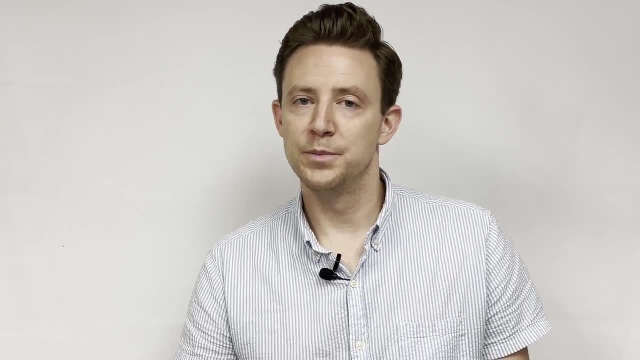 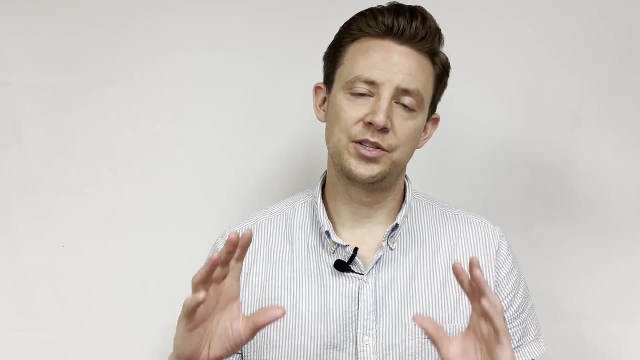 models, visualize data, transform data, perform spatial analyses, understand spatial relationships. You can even create web maps right from QGIS. Like I said, this helps you get started and build some of that basic knowledge in a very familiar and approachable interface. I love the fact that in 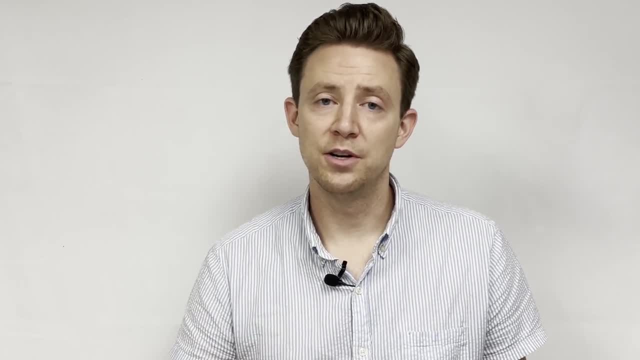 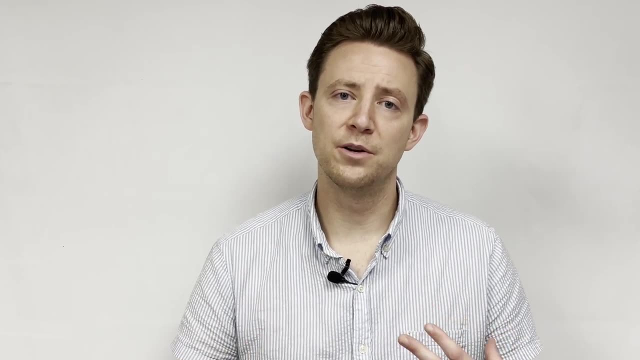 QGIS you can connect a spatial database- use PostGIS or others and connect that and start visualizing it in the tool. One of the toughest parts about getting started with spatial SQL is sometimes, if you're just using a peer database or data warehouse, you can actually see the results. 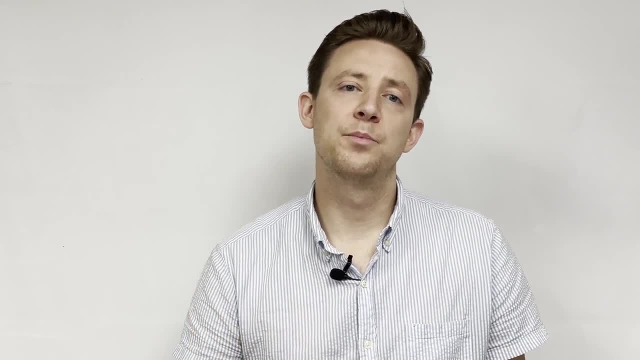 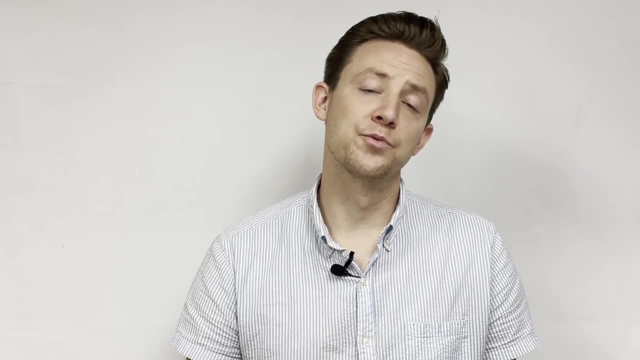 you're producing in the SQL you're writing. QGIS solves that problem by creating a direct connection to the database or the data warehouse and allows you to visualize that data as you write the queries. This is really important and a great toolkit to get started at a really low barrier to 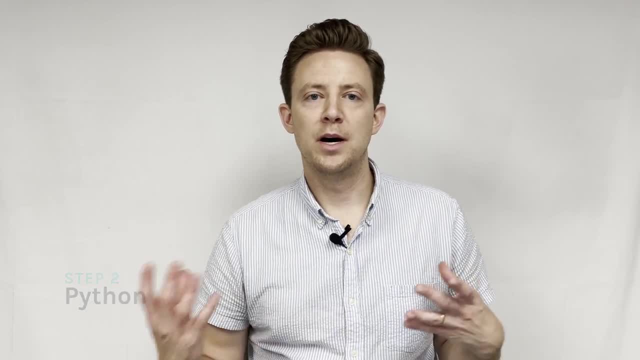 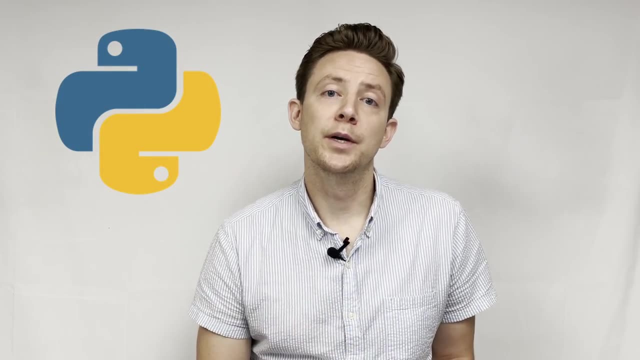 entry. So it seems like we almost can't talk about modern GIS or geospatial data science without talking about Python. Python is one of the fastest growing languages and is one of the most in-demand job skills, whether you look into it or not. QGIS is one of the fastest growing languages and is one. of the most in-demand job skills. whether you look into it or not, QGIS is one of the fastest growing languages and is one of the most in-demand job skills. whether you look into it or not, QGIS is one of the fastest growing languages and is one of the most in-demand job skills, whether you look. 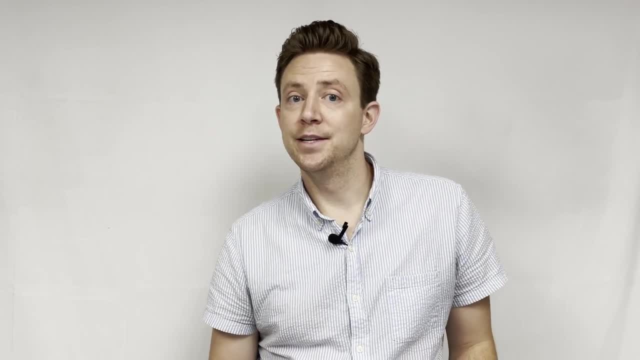 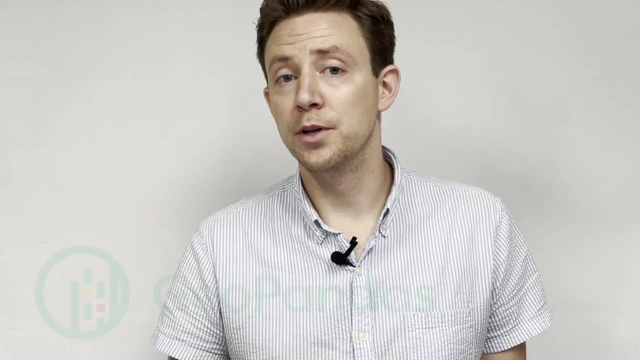 inside GIS or outside of it, into other areas like data science or data analytics. So there's a few core libraries that I think are critically important to modern GIS. One of the first is GeoPandas. GeoPandas has your common geospatial or GIS toolkit to perform. 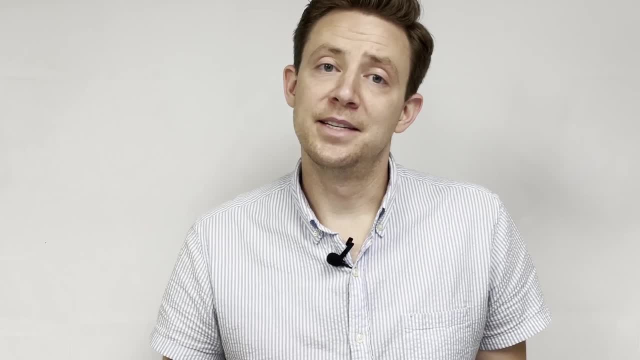 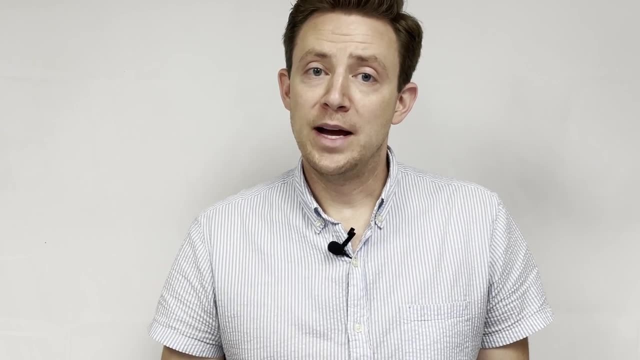 different things like spatial joins, measure areas, distances, intersections, so on and so forth. Has a lot of the core functionality for reading files. Uses a common data format, which is the geodata frame, the common data frame, the common data frame, the common data frame, the. 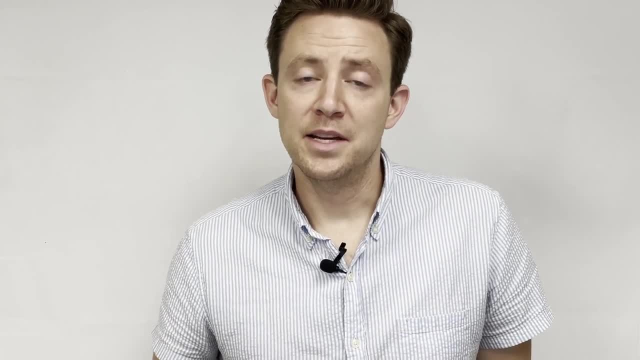 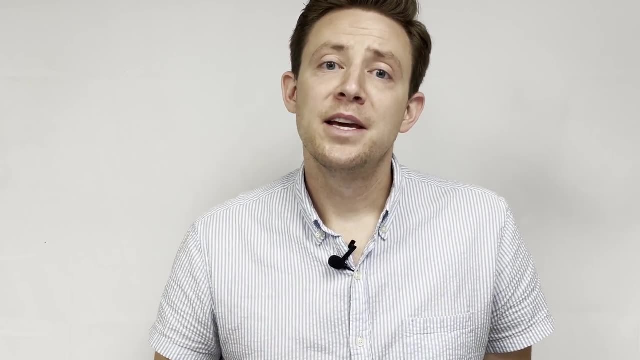 comparable version of that in the non-geospatial toolkit of pandas is the data frame. So you'll be picking up skills to use a generic data analytics toolkit in Python with pandas, and that data frame is transferable across lots of different libraries. Geopandas is actually very easy to learn. 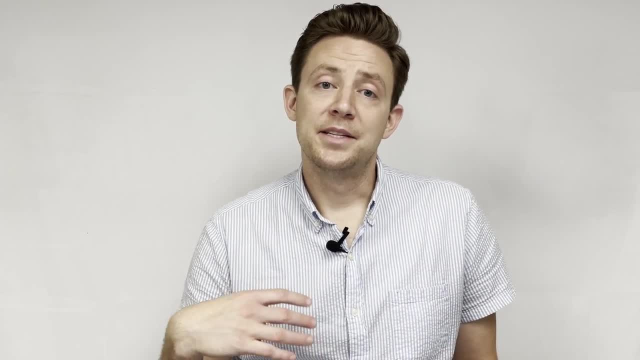 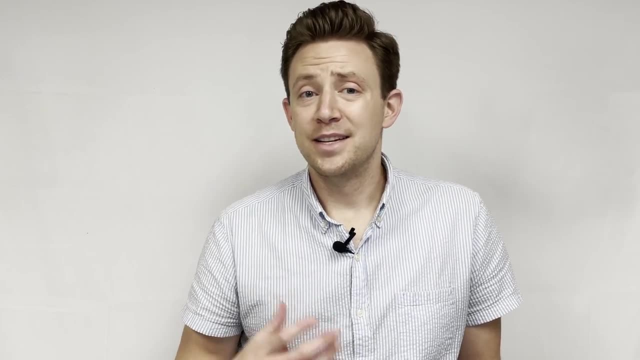 Their documentation is really, really fantastic. It has easy-to-access tools. You can actually click to open up any of their documentation pages directly with a binder notebook and you can get started right now just opening it up, trying it, doing some basic analytics and visualization. 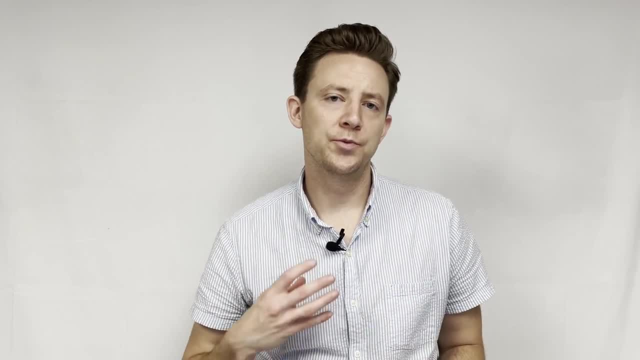 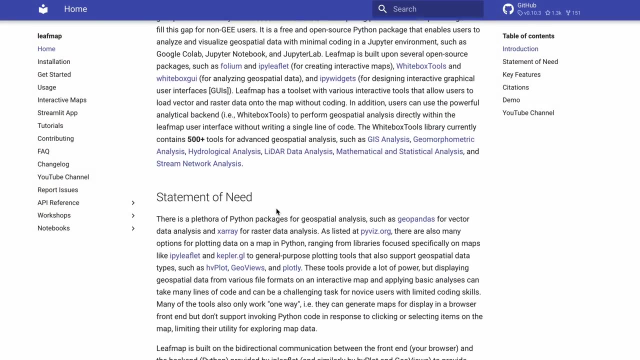 right from Geopandas. So the second toolkit is one that's really starting to gain some traction and I highly recommend checking it out. It's called LeafMap and it's developed by a fantastic professor from the University of Tennessee, Professor Qisheng Wu, and he has built, I think. 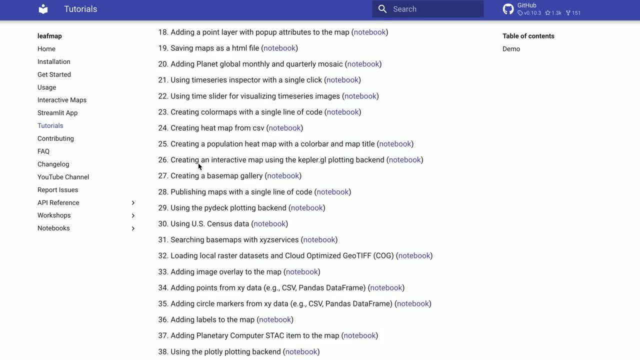 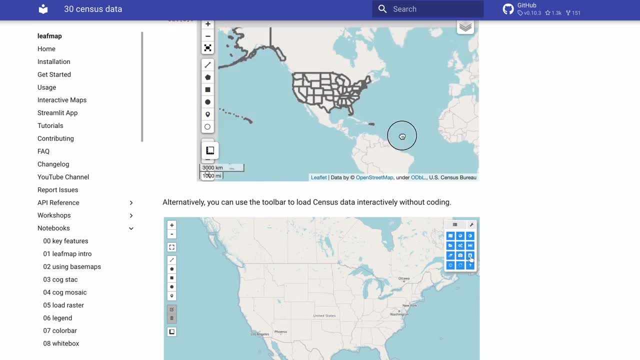 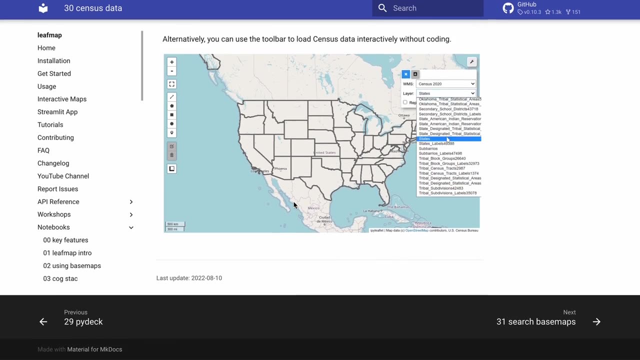 one of the most comprehensive geospatial toolkits in Python that exists today. LeafMap has lots of different tools and incorporates common visualization Libraries. you can use data coming from geodata frames, from post-GIS databases, from just about anywhere. You can perform vector analytics, publish maps and you can perform raster analytics using 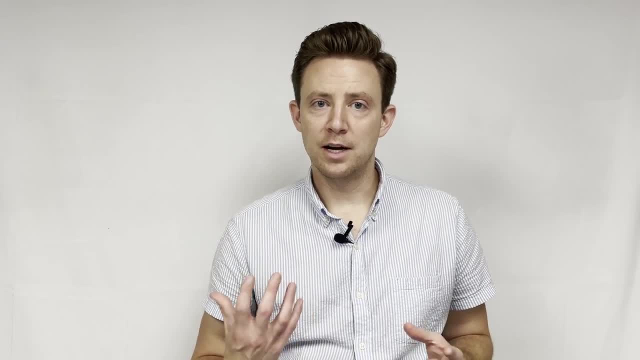 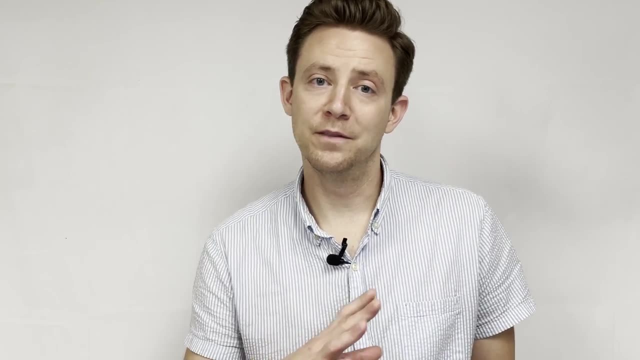 white box tools and many other toolkits. It's really a full, comprehensive, modern GIS toolkit, all written in Python ready to use in notebooks. My favorite part about all of this, though, has to be the examples that he's put together. There's a comprehensive examples library to do. 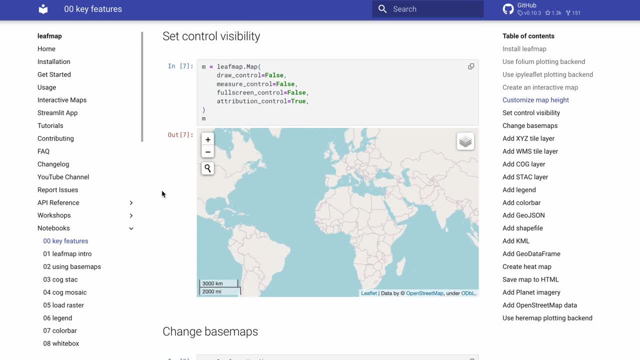 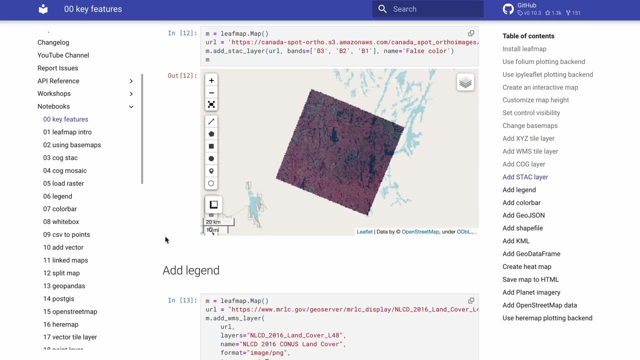 just about anything you might want to do. You can pull the example, get started and start using it today. Like I said, in a combination of GeoPandas plus LeafMap, you can basically replicate just about any geospatial analytics that you might. 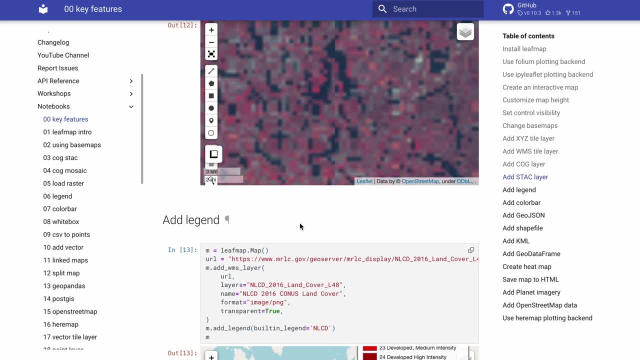 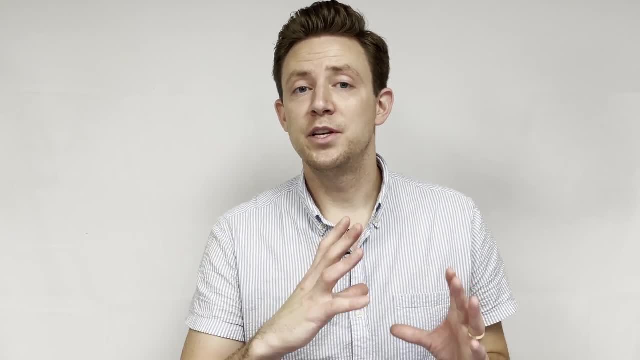 want to perform in a tool like QGIS or any other desktop in a Python environment. Going back to the crawl, walk, run, sprint workflow that I described earlier, starting with QGIS, you can really get a base in modern GIS and some of the tools that you can use there and then making that next leap into 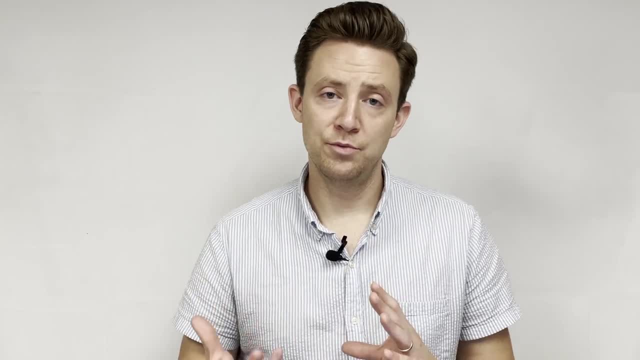 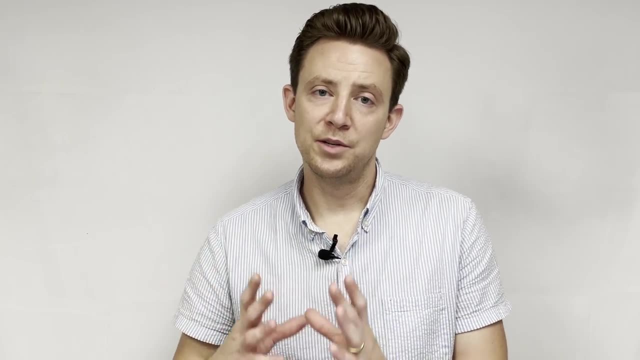 Python. with a combination of GeoPandas, LeafMap and a combination of GeoPandas, You can really start to build that flow. learn what you're doing in Q, translate that to Python, get some of the Python tools under your belt and then make the next leap from there, which we'll 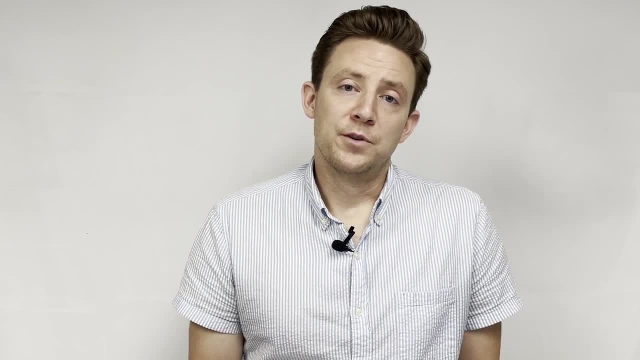 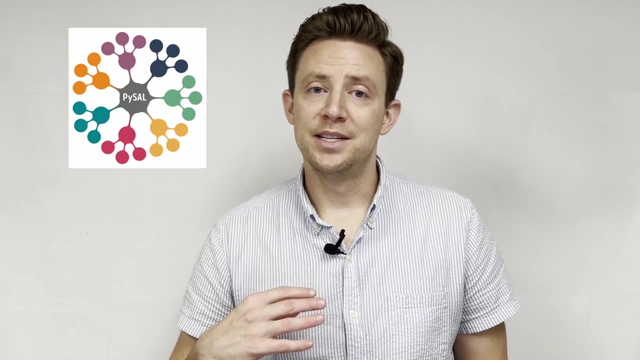 talk about in the next section, The two other components within Python for geospatial that I would recommend would be. the first is PySAL. So if you're doing anything related to spatial data science and really want to get into that statistical modeling and looking at moving from the where to 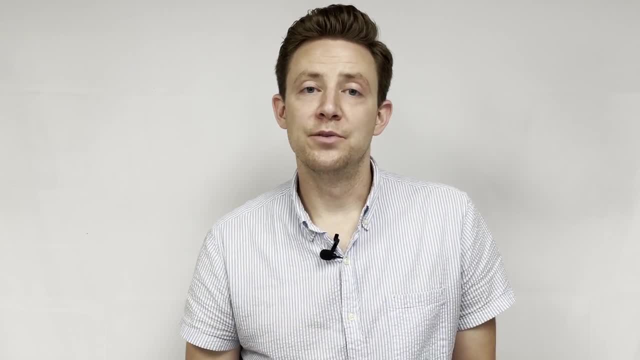 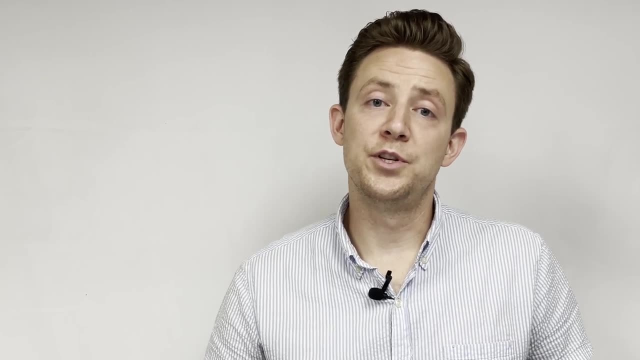 the why things happen. PySAL is absolutely the best toolkit to do this. There's plenty of examples and you can check those out in this video that I'll post it earlier here. If you're looking at doing any sort of geospatial data engineering or want to get under the hood of what's happening, 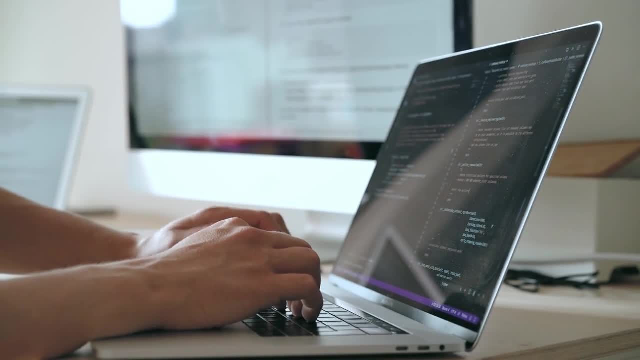 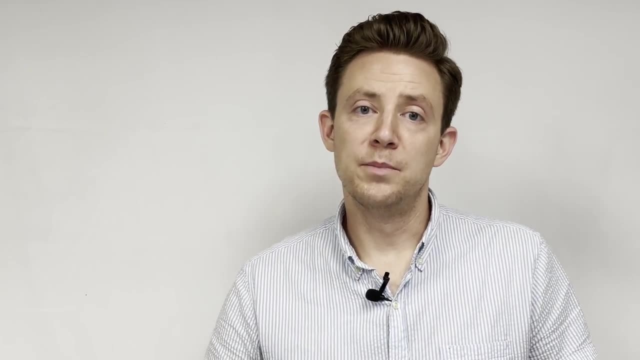 with these libraries, definitely check them out. I would recommend checking out Rasterio for reading and manipulating raster data, Fiona for looking at vector data and manipulating that type of data set, and then the last one is Shapely for editing, changing, manipulating geometries. These are 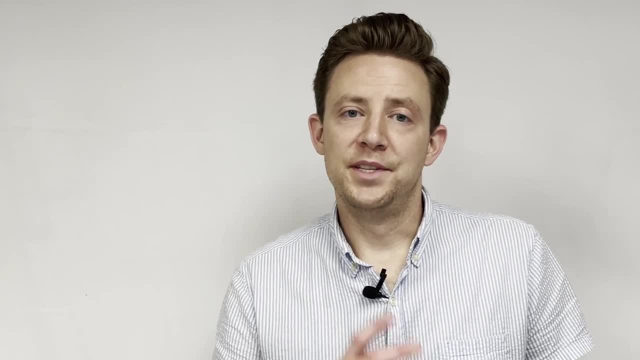 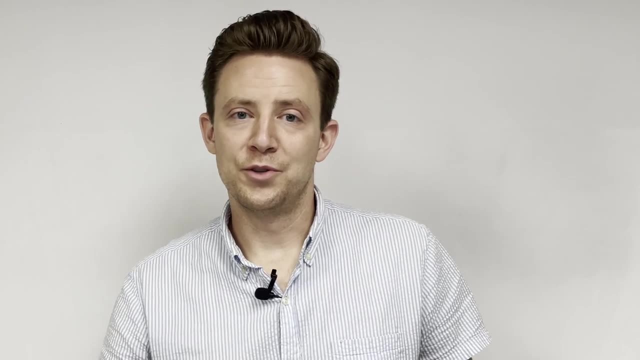 components of geospatial Python, and just about every library out there uses these in one way or another. And one extra note: one layer underneath all these libraries lives our friend GDAL. GDAL, like I said, is one of those core pieces of modern GIS infrastructure that finds itself in just about 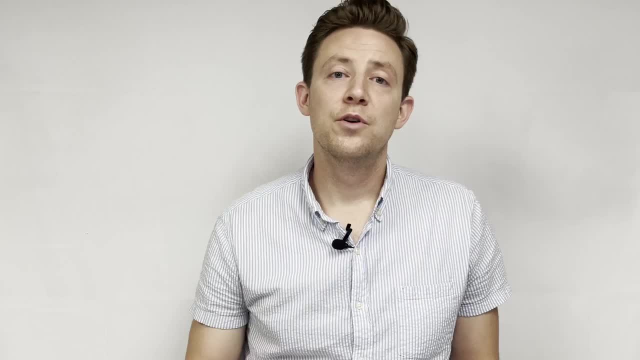 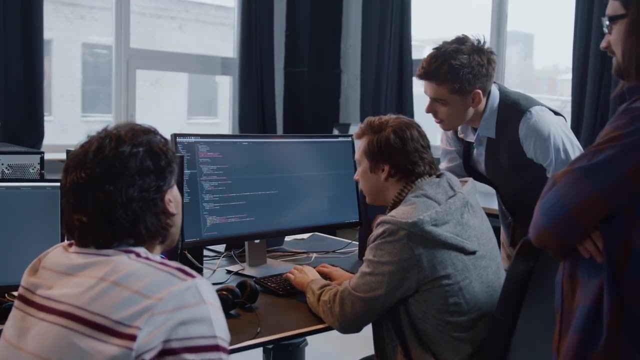 any tool that is currently used within the modern GIS stack. Why is Python really important and why do I push it so much as a second step in the process? One is that you can do so much more with Python, including geospatial data engineering to build data pipelines. 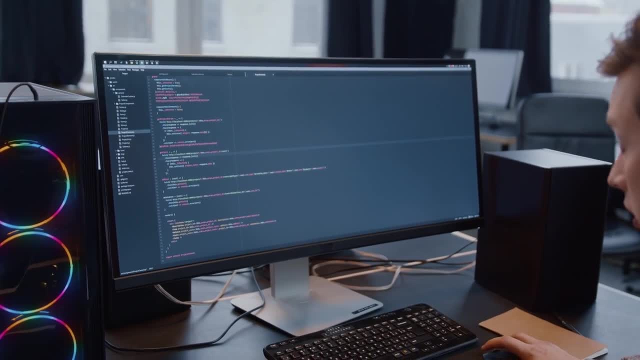 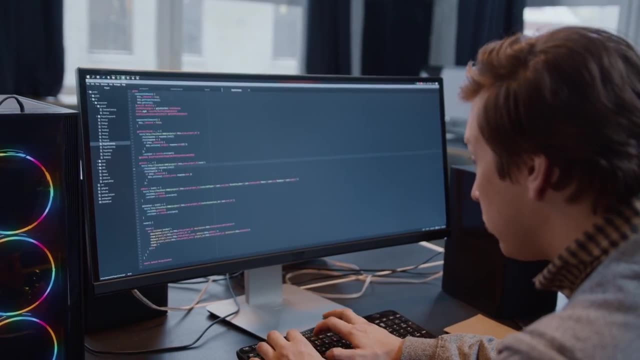 you can use it to read data from APIs and actually create your own APIs and build your own scripts to manipulate data and make processes really repeatable. It has so many uses beyond just the core of data analytics or geospatial data analysis or even spatial data science, that's. 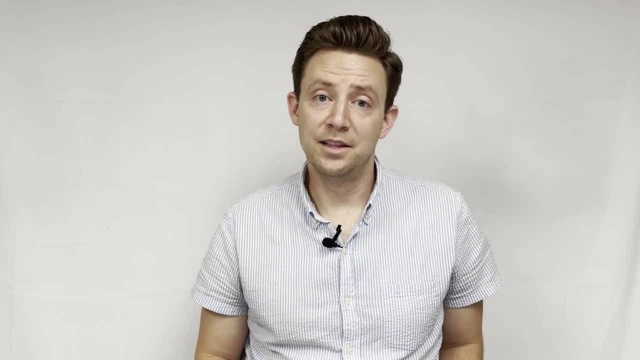 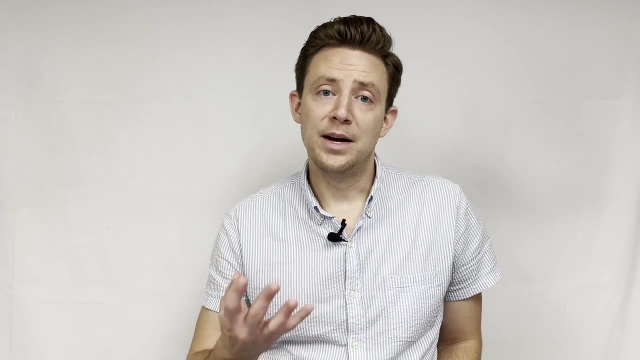 just a good tool to have in your tool belt. Now there's lots of other libraries that I love and recommend in geospatial libraries, like OSMNX and other network analytics tools. we'll talk about those more, but keep in mind I think a lot of these actually read into Leafmap and it makes 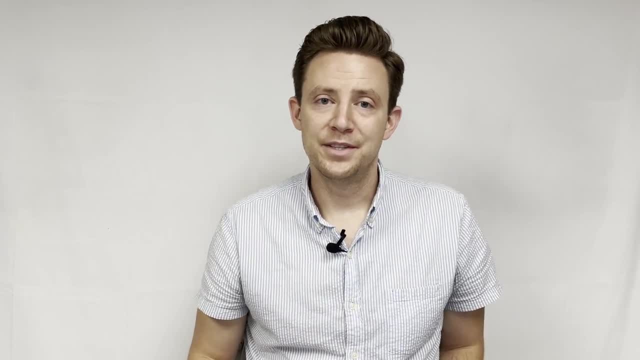 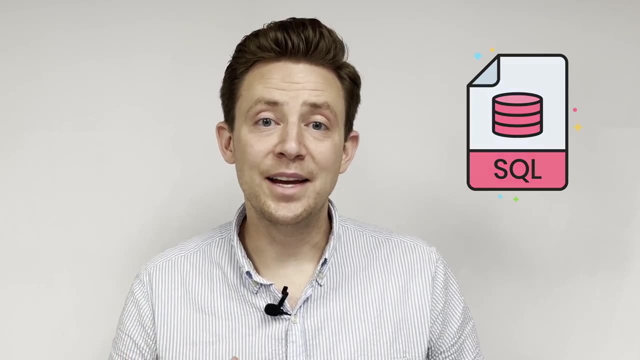 it one of those accessible toolkits that you can use to do a lot of the work that you need to do. If you know me at all, you know I'm a very big proponent of spatial SQL. SQL is one of the first tools that I really started to use to scale up my modern GIS toolkit and I think it's one of 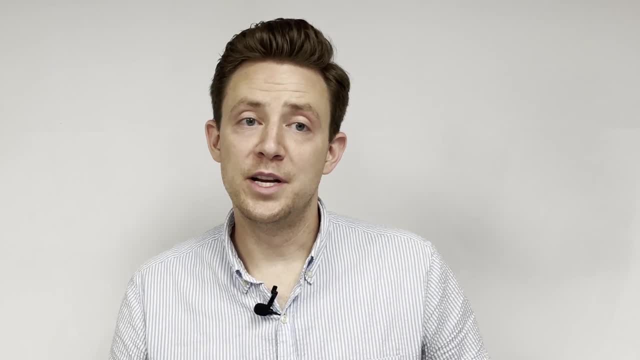 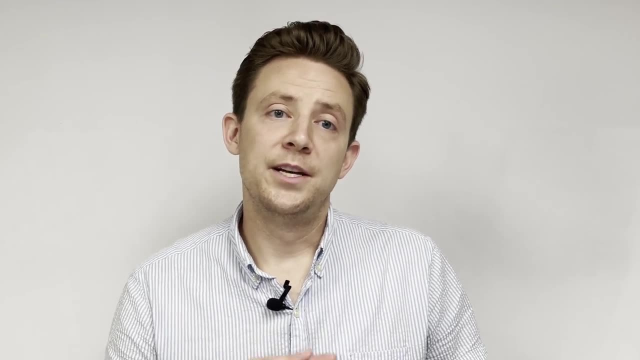 the fundamental pieces that helps you make that next leap. Whether using more data, you need to organize your data in a consistent way, or you want to have a lot of scale and speed to add to your workflows, spatial SQL is the place to do that Now. I recommend adding spatial SQL as the 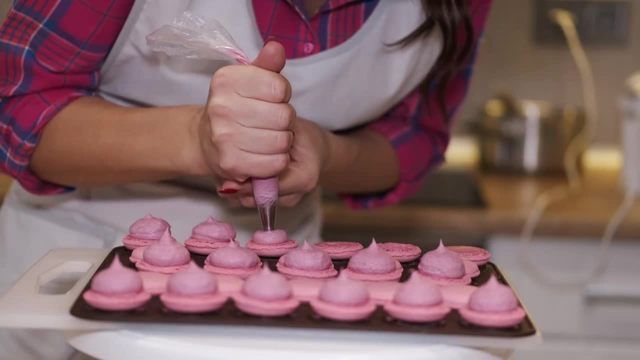 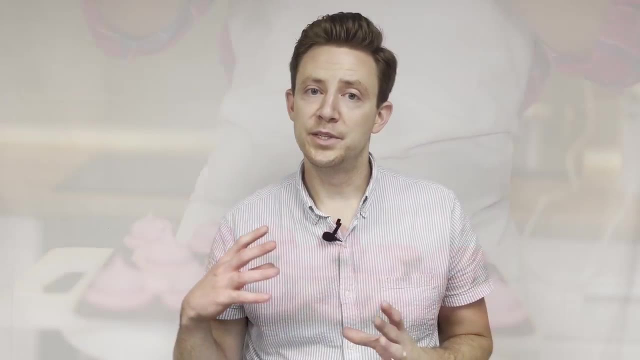 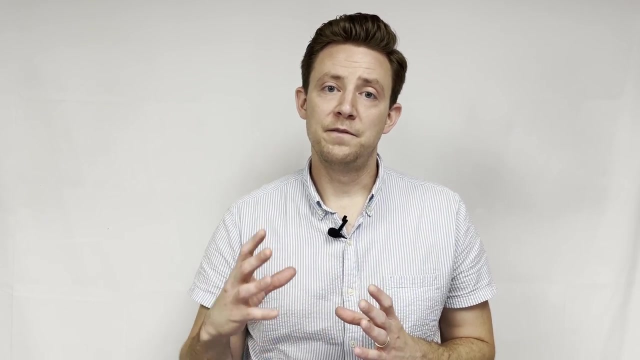 third step in the process. If you think back to the second step of Python, you're translating those fundamentals into a programming or coding environment. Spatial SQL is a different type of programming and you need some skills in computer engineering to stand up a database. or, if you want to use an existing product, do that as well. But SQL adds a few special pieces to your 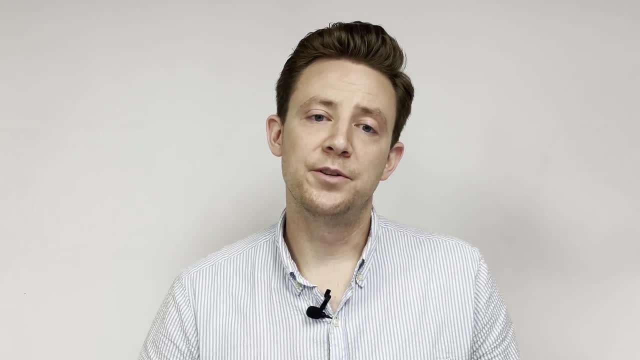 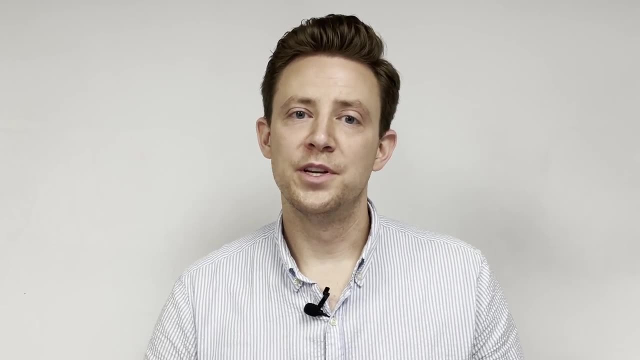 workflow that are really going to help you scale and grow. When you need to use spatial SQL, it's probably around the time when your data is getting a little bit unorganized. you have too many files getting too big that it's really hard, or the processes are taking too long to run in a local. 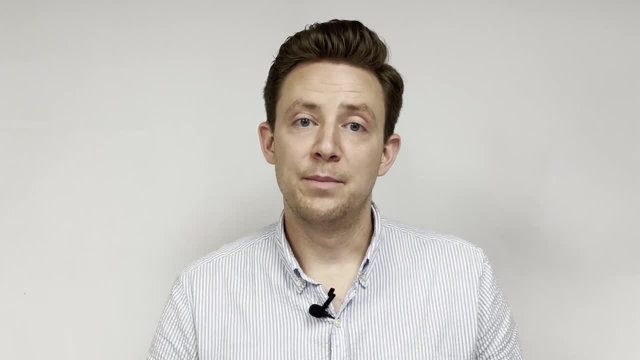 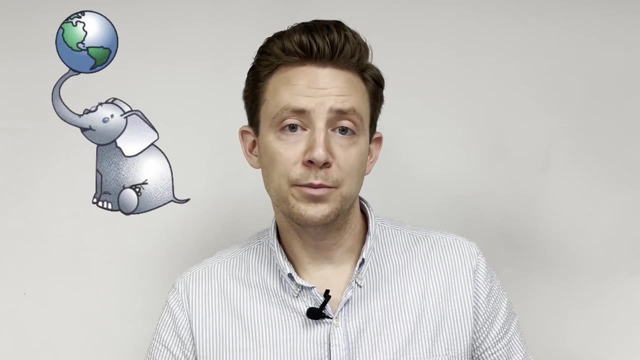 environment or a notebook. At that point in time, you should start thinking about looking at a spatial database or data warehouse. Something like PostGIS is the most common for setting up and you can set that up on your local machine, and there's a couple different ways to do that In addition. 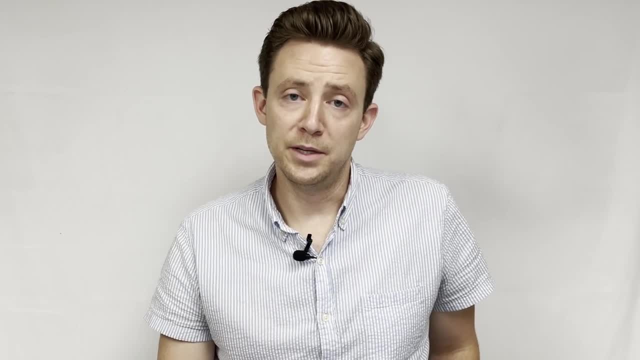 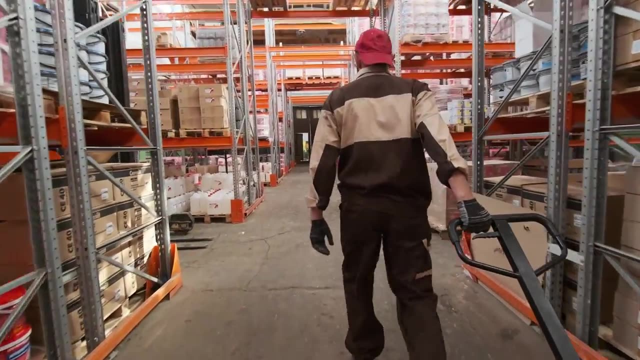 if your data is getting very large in terms of the millions or even billions of rows or complex geometries, I would start evaluating a data warehouse, Something like BigQuery, Snowflake, Amazon, Redshift or even Databricks. These are great tools that are cloud hosted and you can start at a very low. 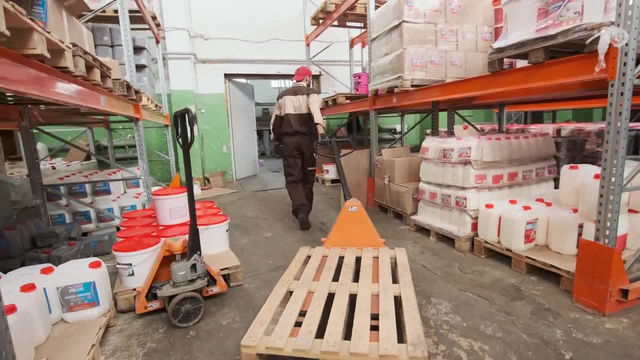 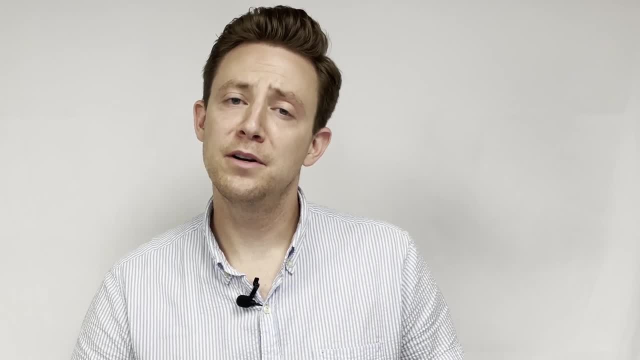 barrier to entry to get started and use those cloud services. So why spatial SQL? What does it actually help you do? Well, there's a few different things and you can check out this video exactly what the use cases are and how that helps you scale. But if your data is getting much larger, 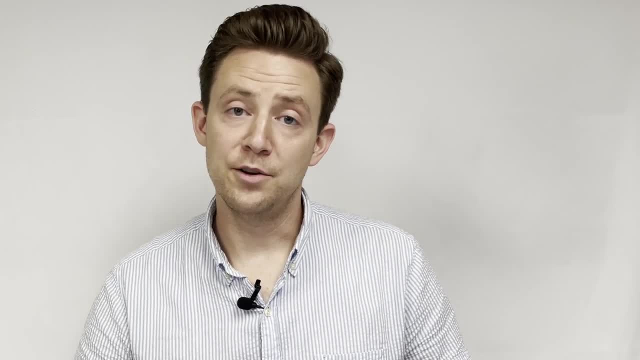 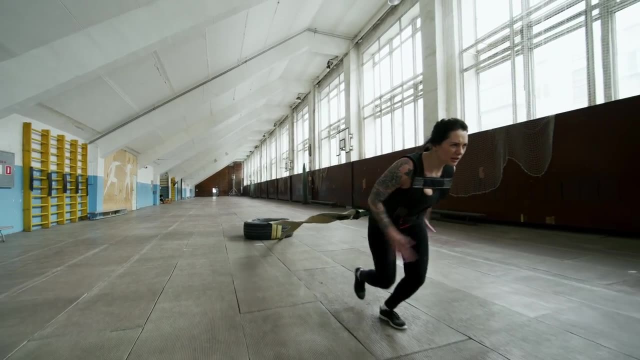 if you're querying more data and you need to maybe create new features or do really large spatial joins, SQL is going to be the best place to do that, Having your data living right alongside the code that's running. it is very effective for creating scalable workflows and you can decrease. 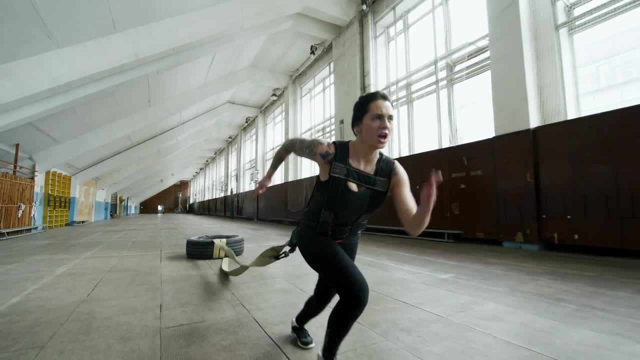 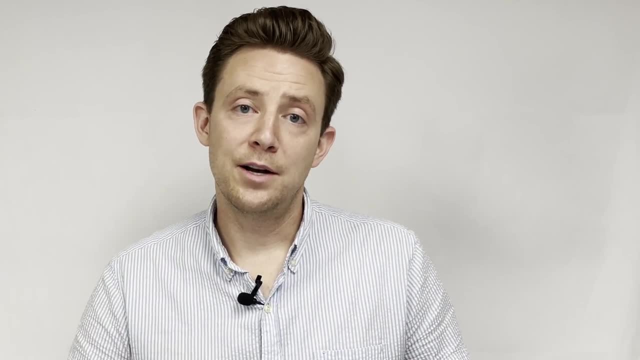 the time you're actually using to perform these spatial analyses, Going back to the beginning of the video. spatial relationship analysis is very, very fast in a spatial SQL database or data warehouse. This is one of the number one reasons I recommend going to a database or data warehouse. 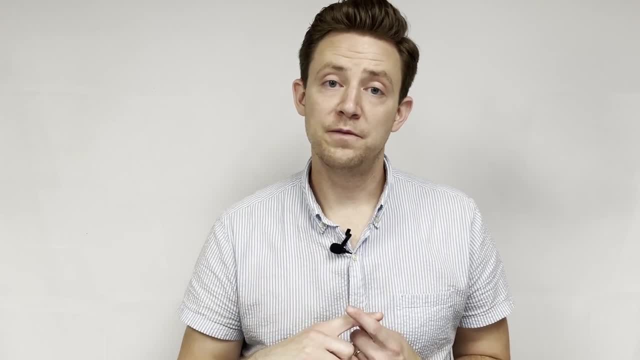 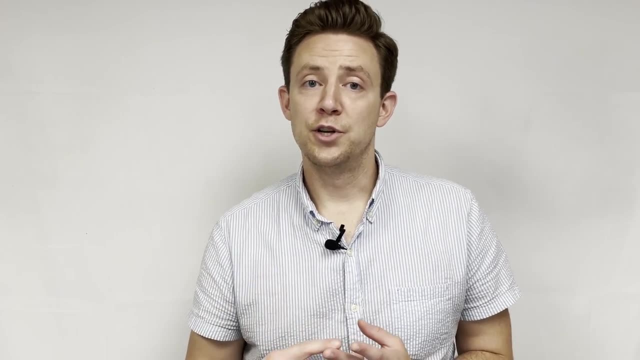 Outside of that, what does spatial SQL help you do? You can do spatial feature engineering to create different features using multiple different data sets in your spatial database or data warehouse. you can actually create tile sets and do visualization from the database or data warehouse too. 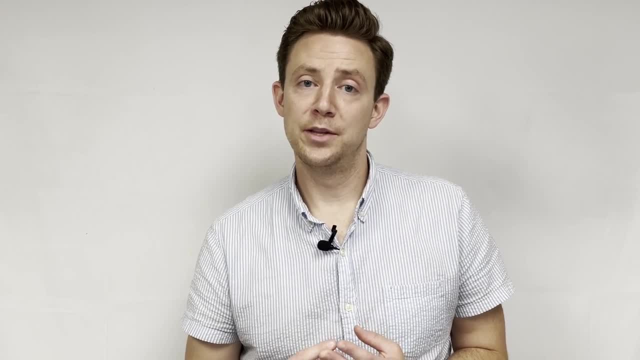 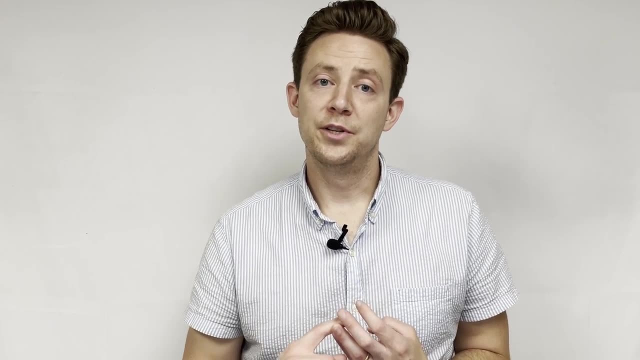 If you have lots of different data and it's better to visualize that in tiles rather than raw files, that's a great place to do that. Data engineering is also much faster and there's so many supportive functions to do geospatial data and engineering. 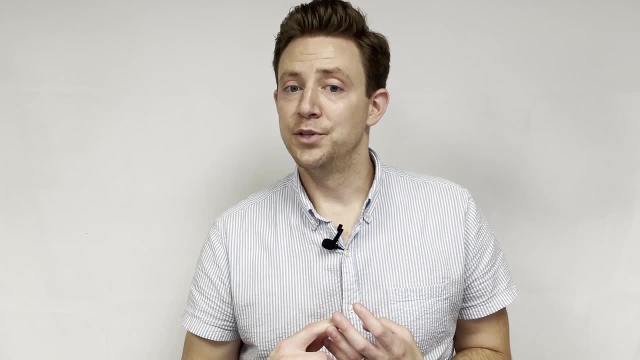 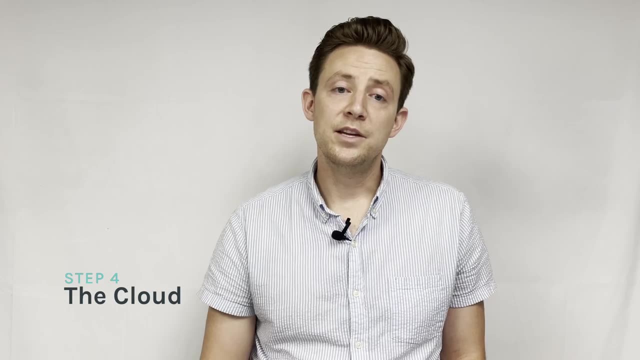 in a Spatial SQL environment as well. I think this is one of the most important pieces in a common workflow. I see people using Spatial SQL for So that wraps up the third step of the process: using that database to help you scale and move into that run workflow. 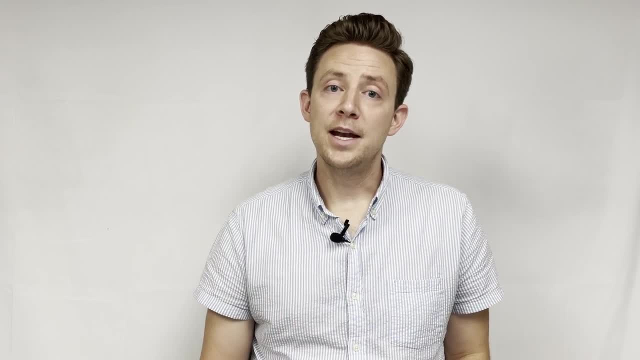 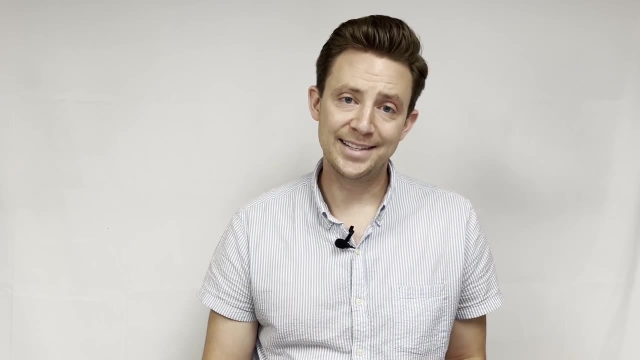 Now, when we're talking about moving into the sprint workflow. any of these first three steps you can run on your computer, in your laptop today. Now, if you're evolving into much larger data sets, larger quantities of data, complexities of data, 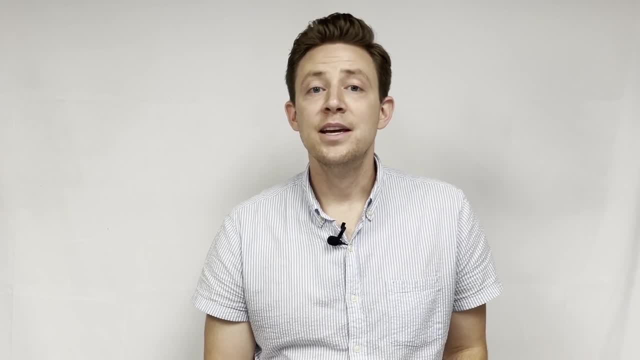 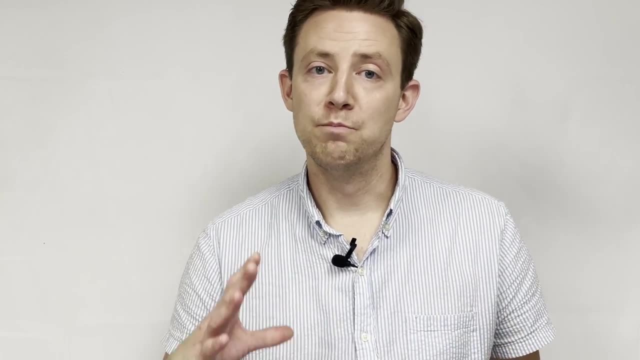 or data that's being added to your data system on a frequent basis. it might be time to think about using the cloud. A cloud is the last piece of a modern JS workflow. It is not something that you must use. You can do all these pieces locally on your machine. 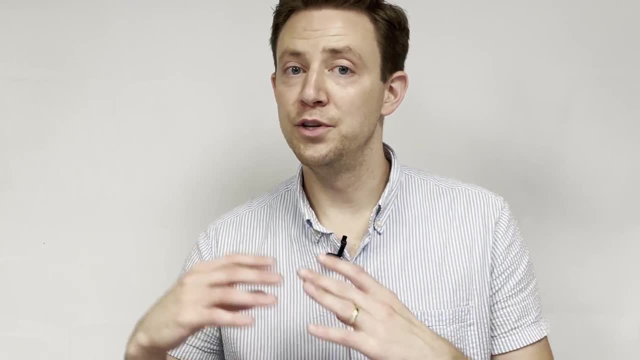 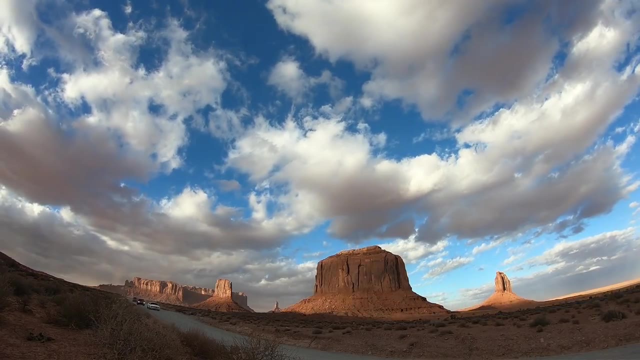 and it's one of the core principles of modern GIS. Anything that you can do in the cloud you can do locally and they're interoperable, But when you're ready, the cloud is there for you to use. Now what I love about the cloud is that it helps you scale. 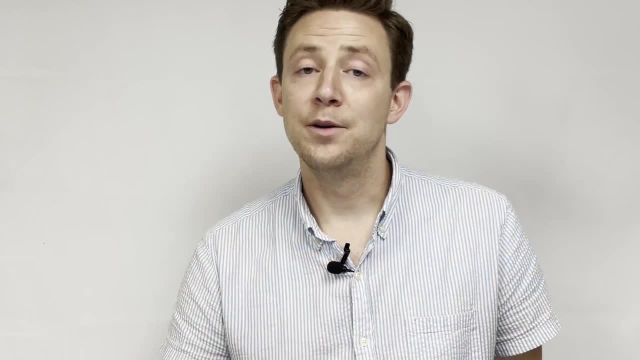 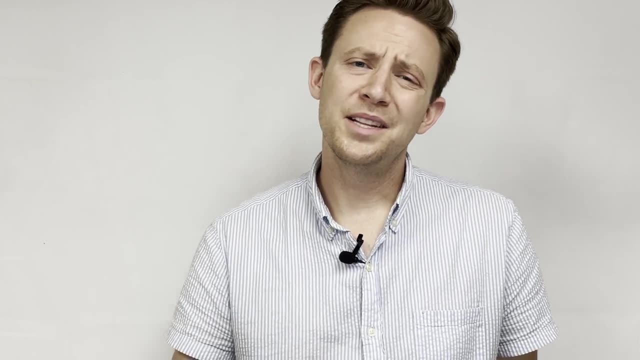 You can do things on machines that are more powerful than what's contained within your local laptop or computer, And you can share that with people around the world as well. But I think the most important thing about the cloud is using cloud-native workflows. These might be known as serverless workflows. 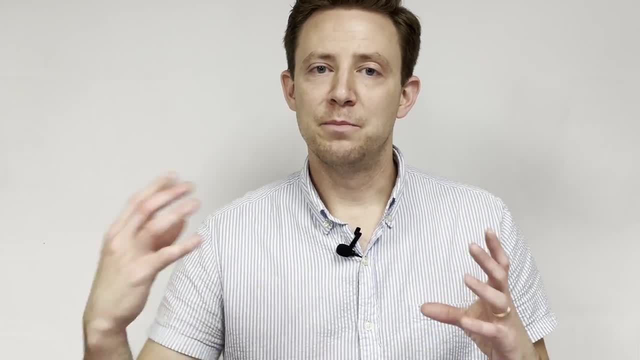 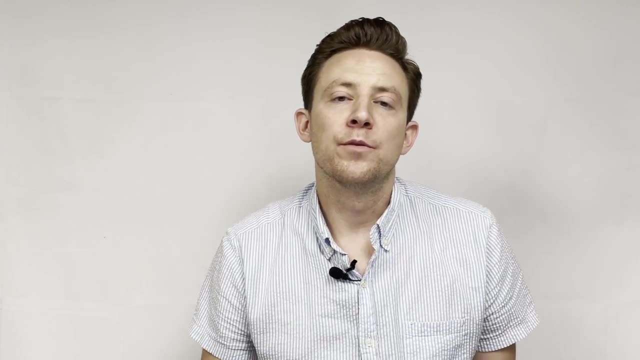 or basically tools that you can spin up and use massive computing power just in the scope of the operation you wanna perform. So what are the key cloud components that you need to use for modern GIS? Well, my top three would be databases or data warehouses. 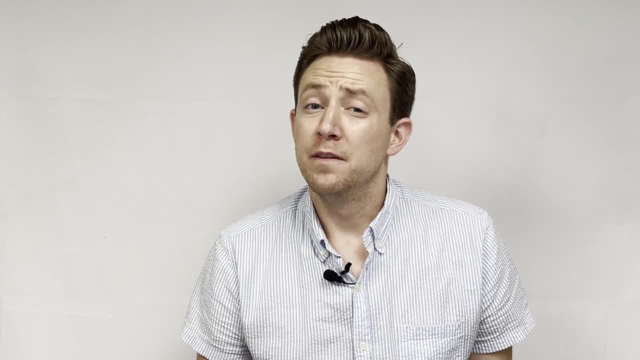 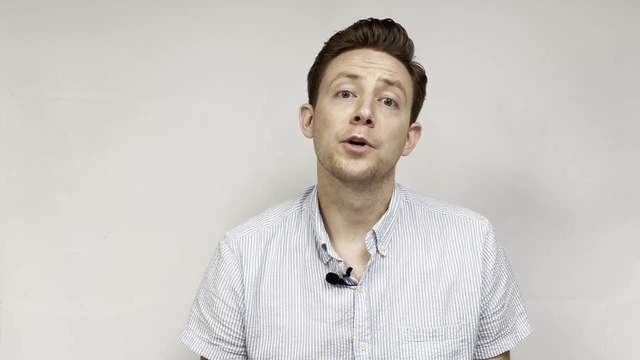 places to store, manage and query your data and do that really efficiently hosted on the cloud. The second would be cloud storage systems where you can actually host and keep your files in an organized fashion. Now this really helps and is commonly known as a data lake. 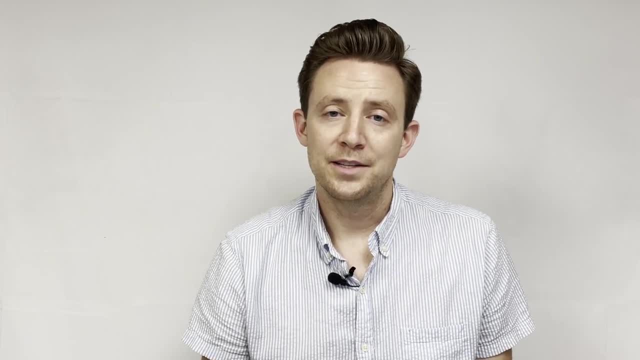 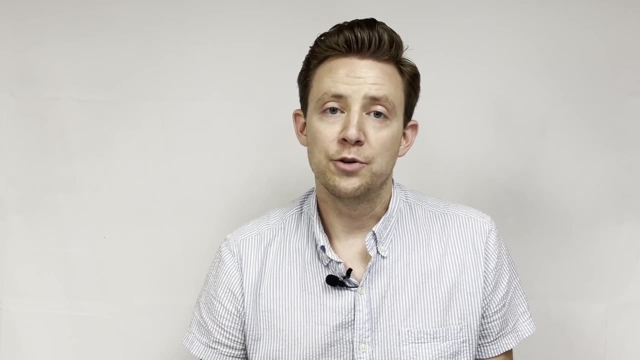 but effectively it's a giant storage system to keep all your files organized. The next would be ETL or ELT tools to actually load data in. This could be products that stream a batch or are streaming data into a database or data warehouse. 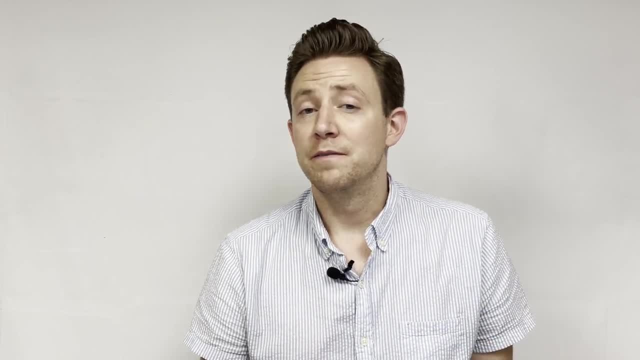 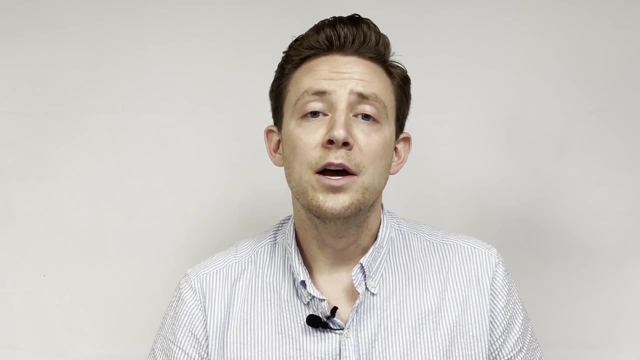 but provide that serverless layer that I was talking about earlier to make that really efficient and effective. There's lots of tools to do this, but definitely not time to cover that in this video today. Some of the other tools that I would take a look at. 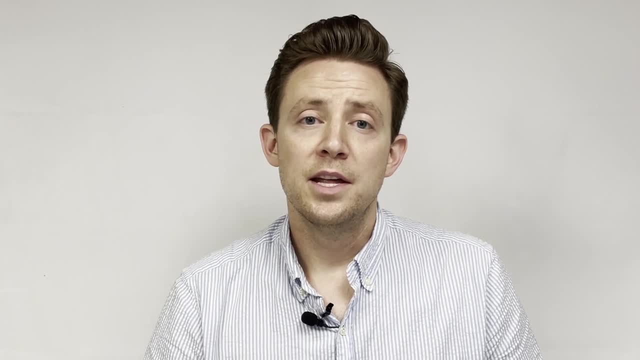 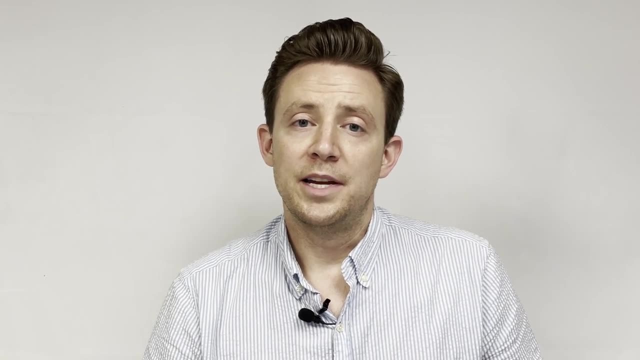 would be notebook services where you can actually run hosted Jupyter notebooks, things like APIs for maps or mapping applications and several other components that are helpful within the cloud stack as well. The last thing that I would have to note would be hosting and using Earth observation. 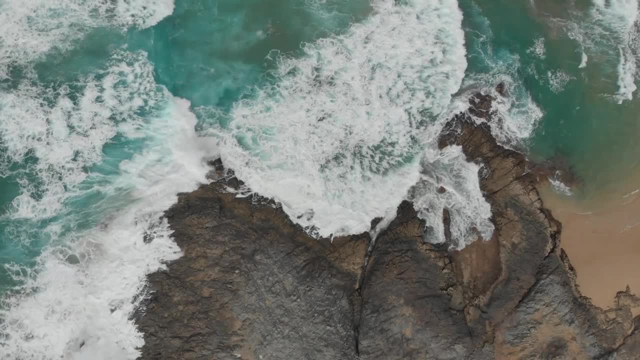 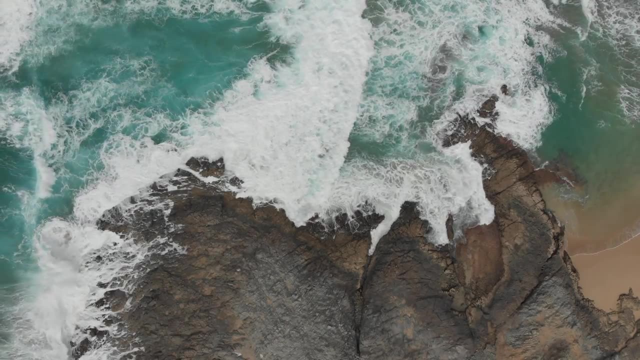 or satellite imagery data. Now, you can't mention that without mentioning Google Earth Engine, which is a really great tool to actually access, analyze and run models on top of historic and current imagery within the Google Earth system. So, now that I've covered those four key areas, 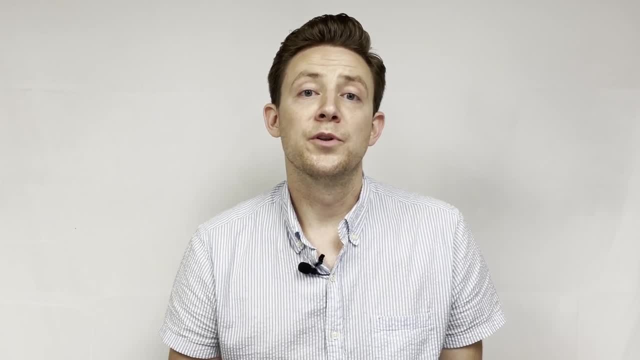 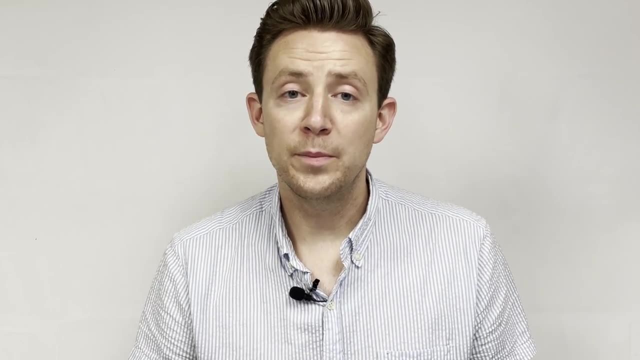 for the crawl, walk, run and sprint. I wanna cover a few other areas that might be important. if you're studying different topics in modern GIS, Using a command line for this first time can seem quite overwhelming and you might think you need a background. 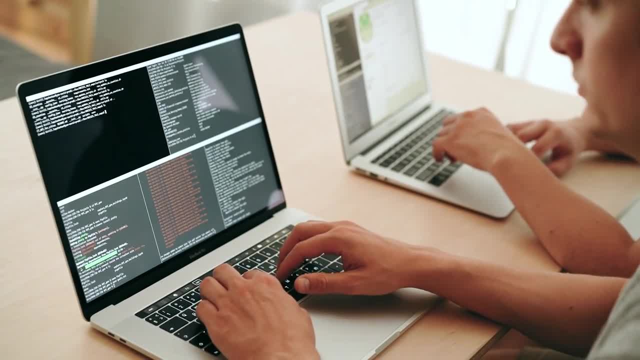 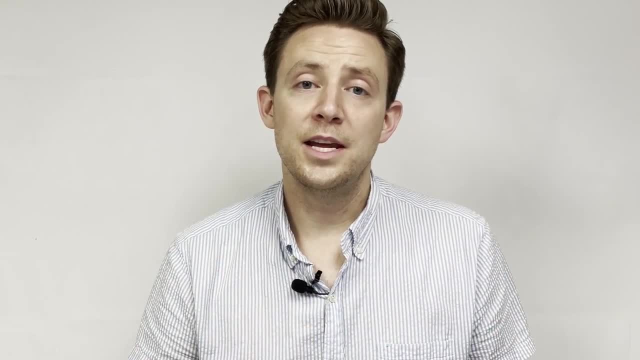 in computer science, but having a complete computer science degree or background isn't necessary for modern GIS. That said, those concepts don't hurt, and there are some great courses out there. I've actually taken the first part of the Harvard CS50 course. 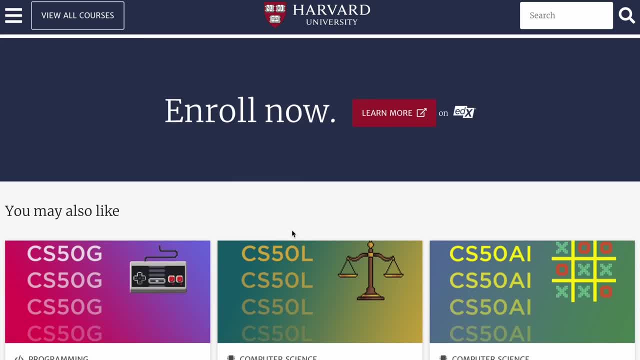 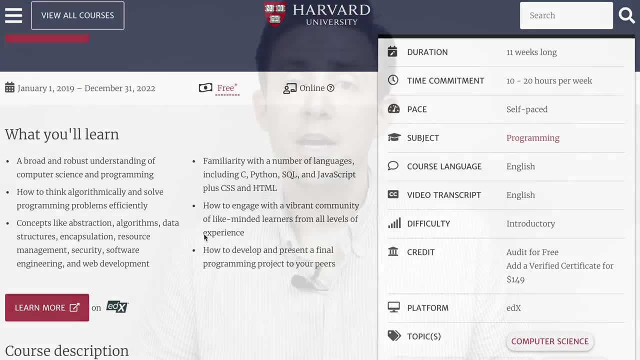 I really enjoyed this. It gave you some fundamental understanding of how computers and programming works, without going too deep or too intense into the topic. Command line is obviously a great tool to know and use, and one I definitely recommend investing some time in, and there's plenty of great tutorials out there. 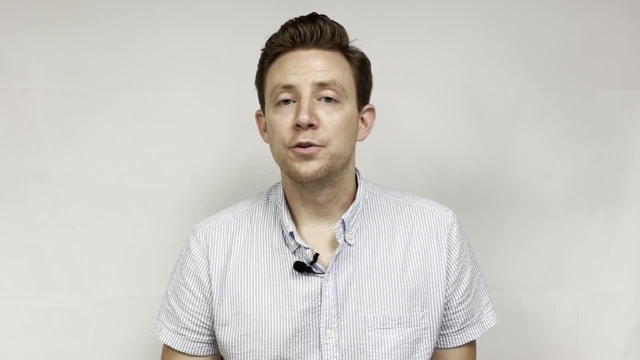 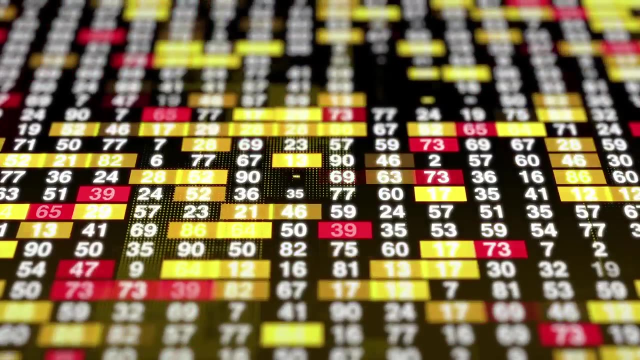 to get you started. The second is basic data structures. Knowing not only data types- things like integers, booleans, strings, dates, geometries, of course are really, really helpful- but having that basic structure of other data types. 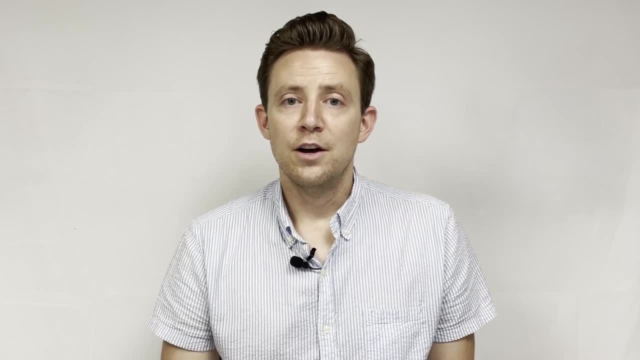 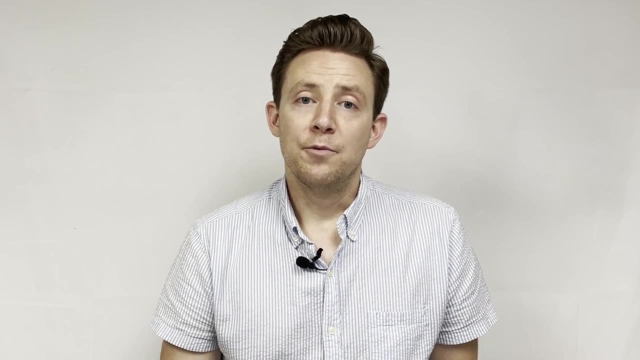 things like JSON, dictionaries, lists, arrays- all these different topics are really really helpful as you start to use and advance data structures within your modern GIS. I really recommend spending some time doing this, but being an expert on it is not necessary either. 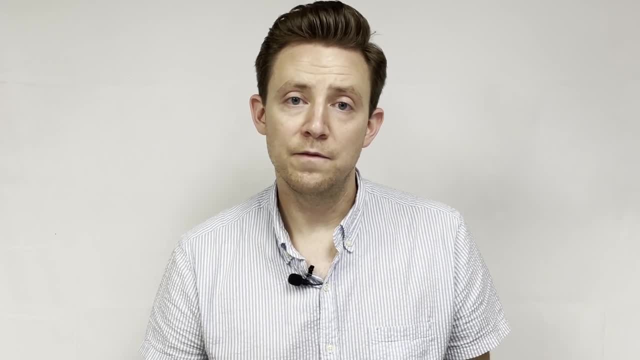 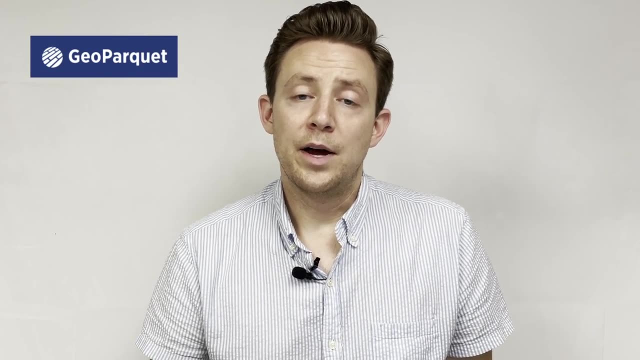 Speaking of data, there's been a surge in creating cloud-native data formats. This includes vector data with file formats like GeoParket, and raster data with file formats like cloud-optimized GeoTIFFs and SARS, among others. Now, I would definitely recommend checking this out. 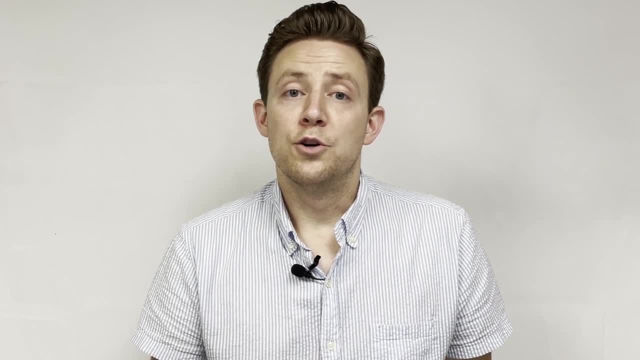 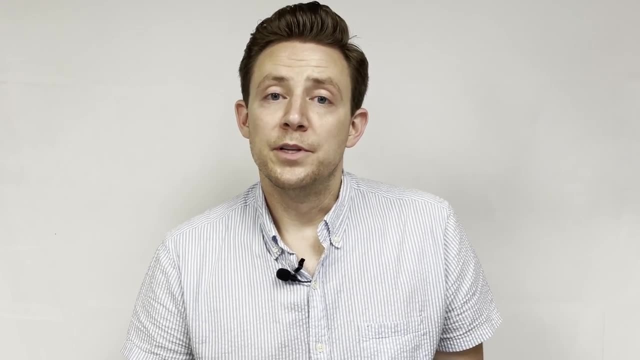 This is a very new and advancing topic, but this video by the Open Geospatial Consortium, which is actually a video of a complete conference, shows some of these different advances, both in the space, as well as some of the use cases you can use with it. 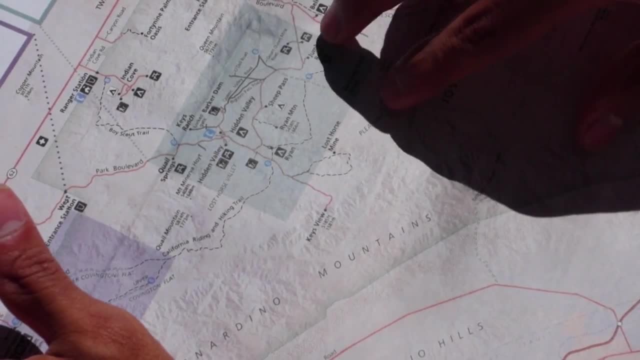 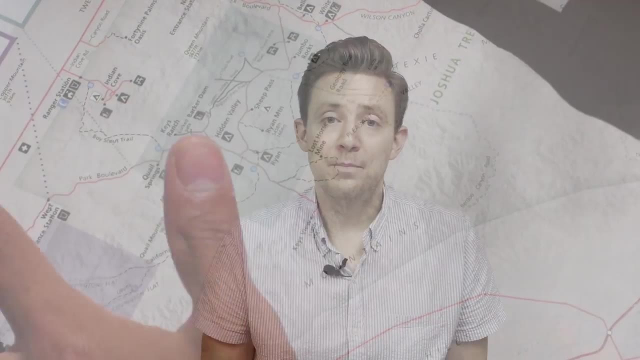 Now, while it pains me, as I have a traditional geography and cartography background, to say that visualization might not be the top of the list for modern GIS skills, the field has advanced quite a bit and with a lot of out-of-the-box tools. 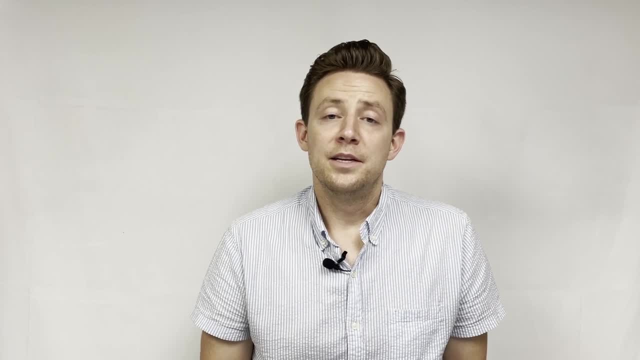 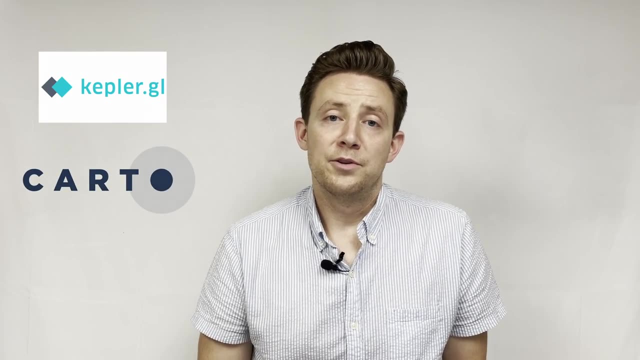 you can build some really great cartography styling and different components into your maps. So tools like Coupler, GL or Carto have really great styling patterns that you can use to create choropleth, categorical maps, as well as a lot of other things you can do with them. 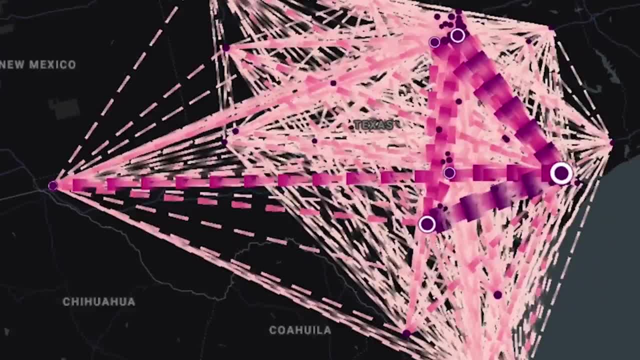 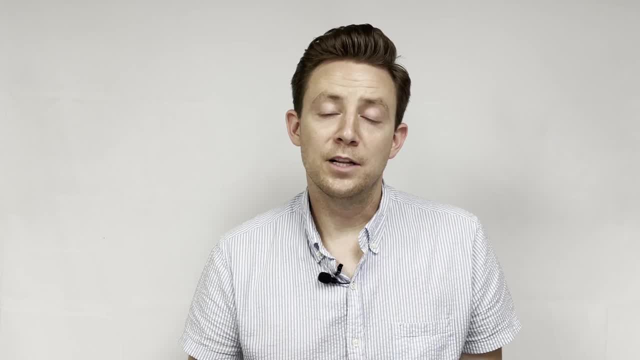 So, while cartography is, of course, really important to communicating what you've done, you have a lot of tools that help you do this. today, If you're doing geospatial application development, of course you're going to need some JavaScript. 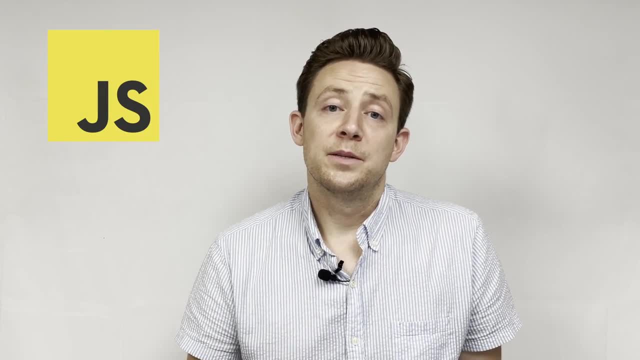 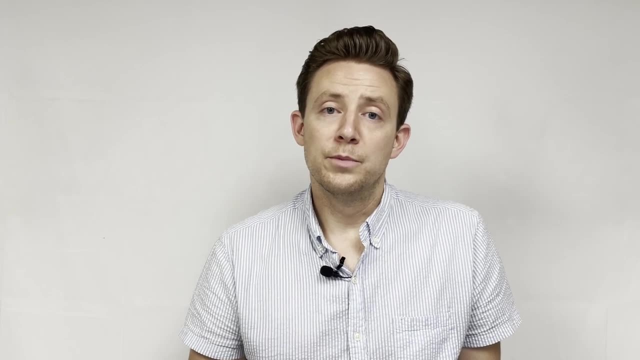 And I also recommend spending some time learning React and Redux as well, as it gives you a really base framework to build and create repeatable components if you're building large-scale applications. Now to advance your JavaScript skills, if you have some basic understanding of JavaScript. 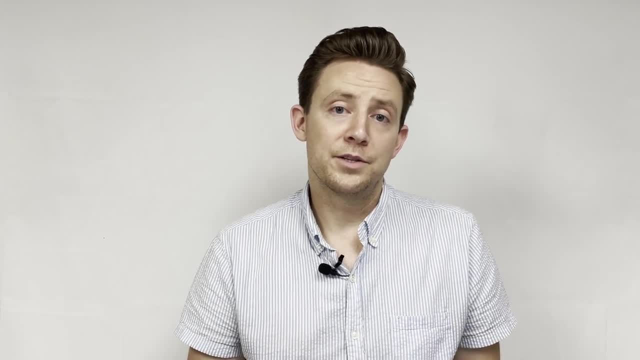 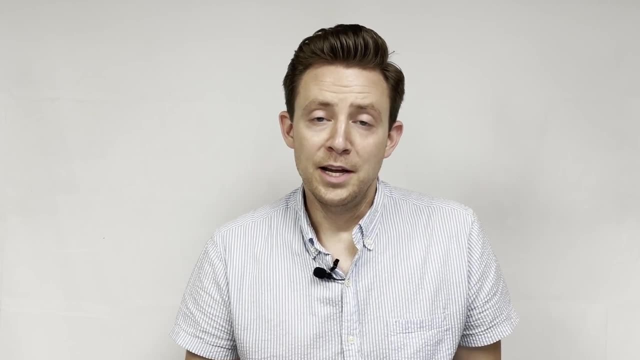 you can use this tool. Understanding of JavaScript. I really recommend this course under Udemy. This is the one I use to really advance my JavaScript skills and really leapfrog into really understanding what I was writing, not just kind of following some tutorial. 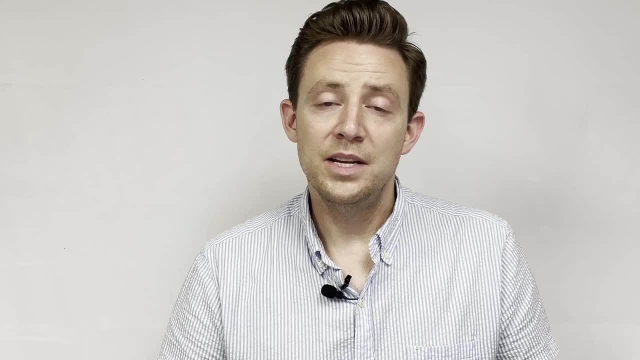 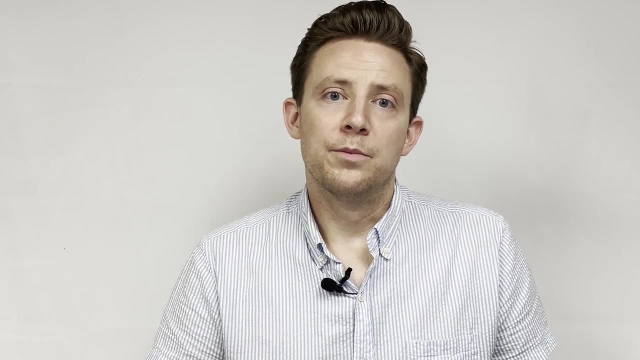 The second is React. I love React and I think it's one of the pieces that I've picked up over the last couple of years. It's really helped me build really scalable applications, make my work way more repeatable, and it's well worth the investment. 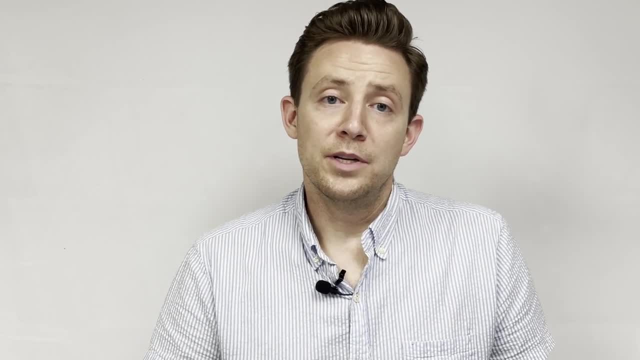 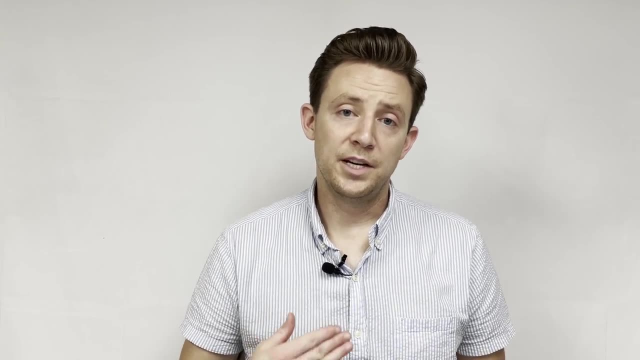 This is another great course from Udemy that I recommend, that I actually helped you use Learn React and Redux, So definitely take a look at this one as well. So the last topic in terms of big data visualization, I have to mention tiling. 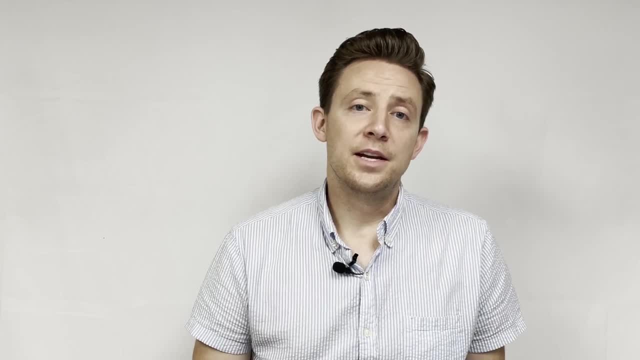 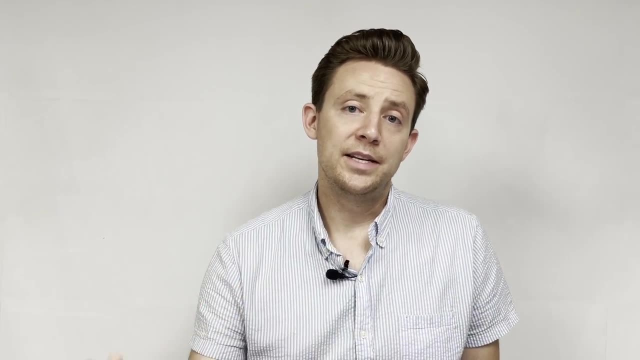 Now, map tiles are the services that we use to render data on the web very efficiently. Effectively, every base map service- Apple Maps, Google Maps- uses a tiling service to render that data. Now, if you don't know anything about map tiles,